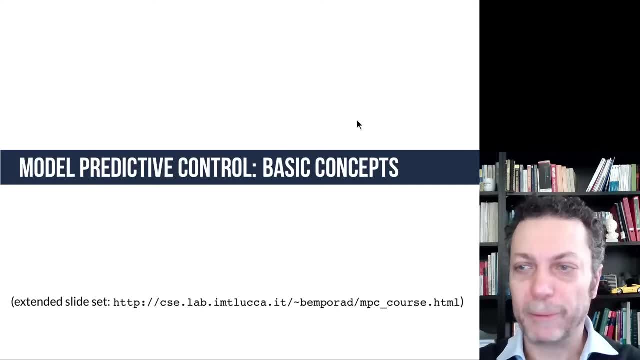 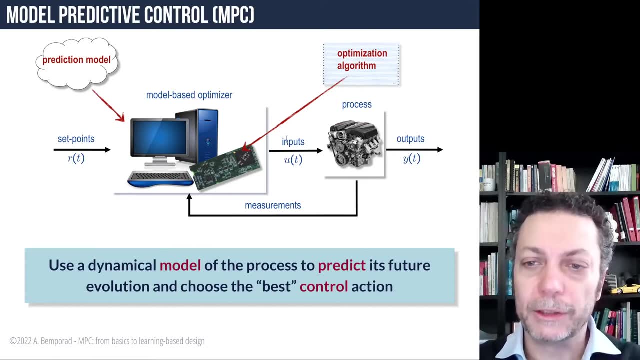 So let me start with the basic concepts of MPC. So MPC is a control technique. So, as every control technique, the idea is to generate inputs to actuate a process, so that the outputs of interest of the process track a certain set point or reference signal. And we want to do this in closed-loop, so by updating. 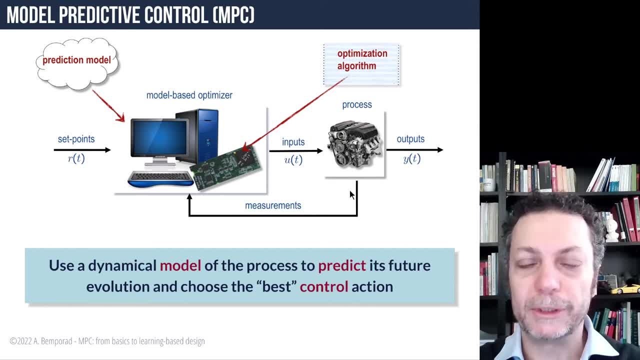 the decision on the value of the input variables based on measurements from the system. Now, the particularity of MPC is that the controller is using express input. That is an expression of a value input variable. So the ratio of the value input variables is a value of the. 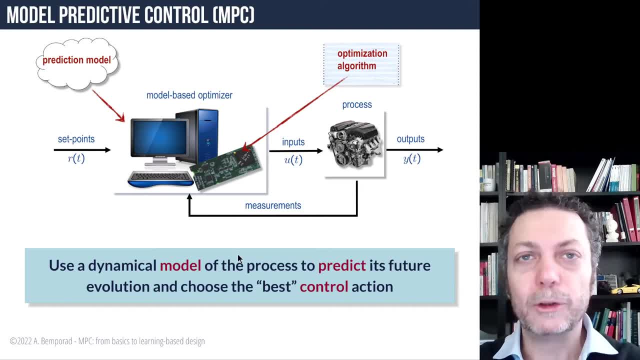 explicitly a model of the process that we are controlling to make predictions of what the system will do if we apply certain sequence of inputs in the future, and by means of an optimization algorithm, the controller will choose the best sequence according to a certain performance index that we'll specify in a second. 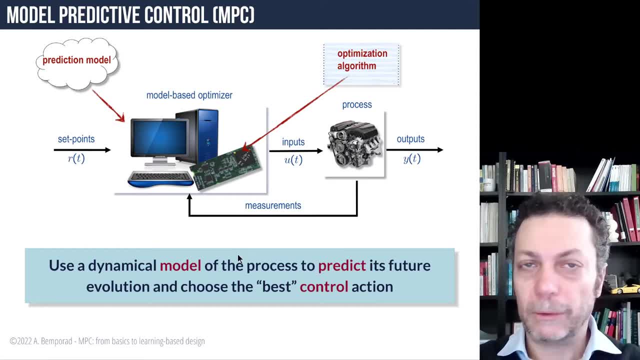 That's why it's called model predictive control, So we're using a dynamical model of the system to predict what the system will do in the future if we apply certain control actions and then, as a result, choose the best control action by means of optimization. Now, in reality, what you do is to: 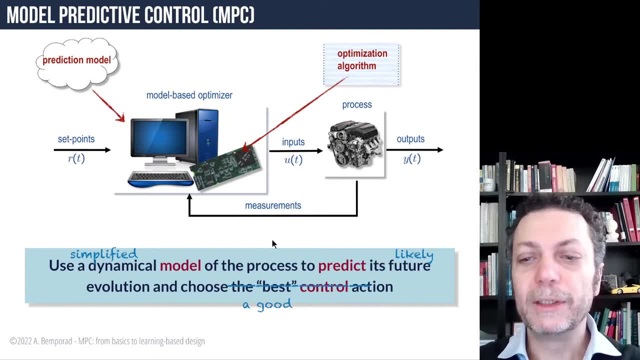 use a simplified dynamical model of the system so to predict what is likely the system to do in the future and, as a result, maybe we don't apply the best control action, but we still apply a good one, and the better is the model we make of the process. 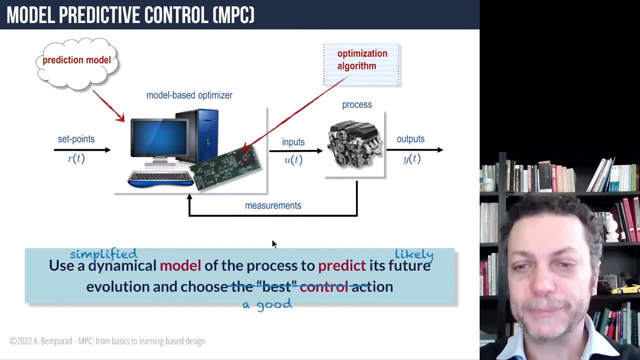 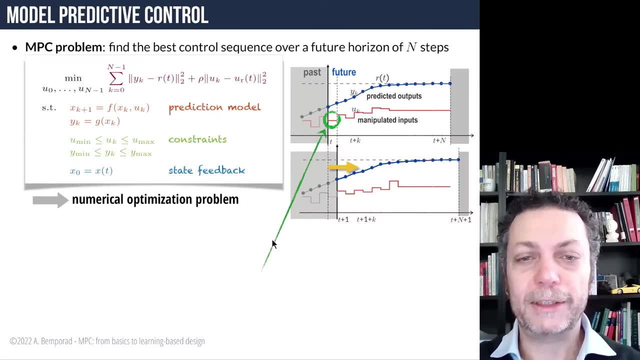 the better would be the control action we apply on the system usually. Now let me state this in mathematical terms more precisely. So say, now is the current time t. We have a certain set point, R of t we want to track and we look at this optimal control problem, finite time, optimal control problem over the horizon between t and a certain time, t plus n. 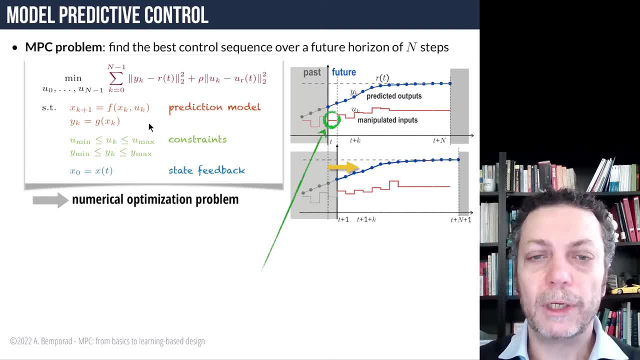 in the future. So what we want to minimize is: what is the tracking error? Okay, this may have different form, we'll see some. in general, you're waiting the difference between the predicted output and the reference. you want to track as well as you have. 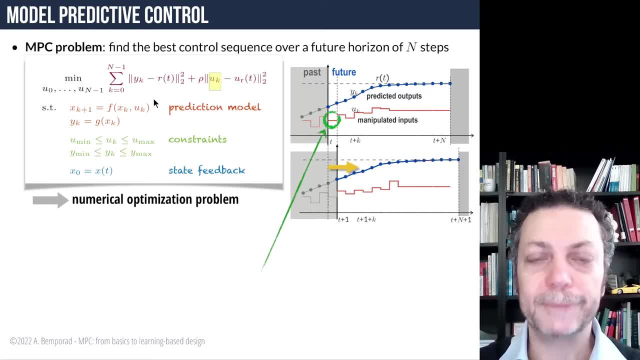 penalties on the inputs that you are applying. So, for example, this can be the sum of the square tracking errors and the sum of the square differences between the input that we apply and an input which is optimal for the reference signal that we are, but we want to track a time t. 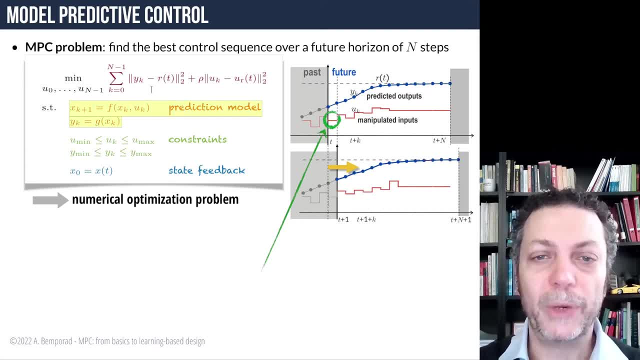 Now this problem depends on the model. So the way the output evolves over the prediction horizon, it depends on the prediction model we're using. so the way we are relating input- applied inputs- to output depends on this model. and one ability of MPC is to include constraints. So if we have constraints, for example, 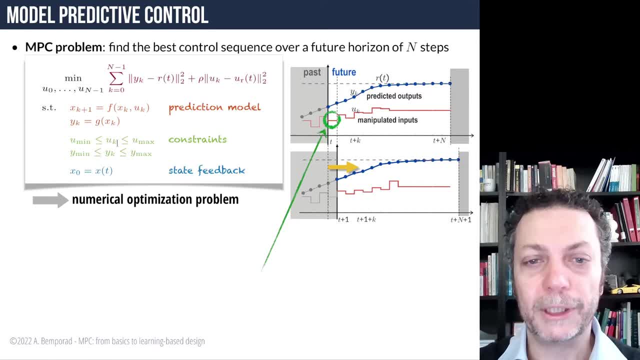 the actuators are limited between a lower and upper bound, then we can include those constraints in the formulation of the optimal control problem, as well as output constraints. For example, we want to keep the output within a certain band of values, Okay. and of course the optimal control problem requires an initial condition. 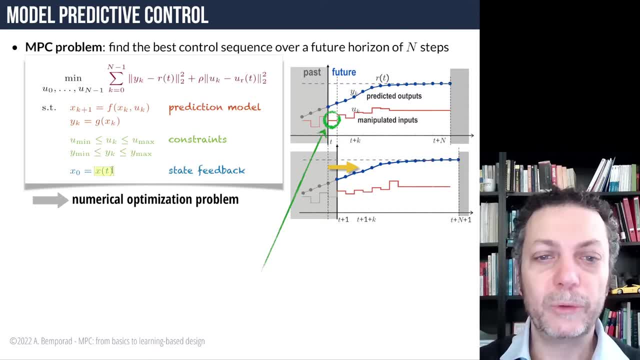 which, since we are optimizing between t and t plus n, will be the current state x. Now let's say we know how to solve this problem, which we will show we can solve. by means of numerical optimization, We will get an optimal sequence of moves, for example the one here depicted in red. 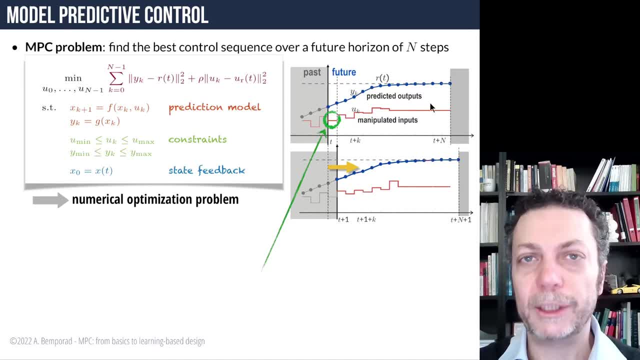 Now what we do. we don't apply the whole sequence in open loop, but we only apply the first sample of the sequence. Why? Because at the next time step t plus 1, we repeat the same process. So we look now between t plus 1 and. 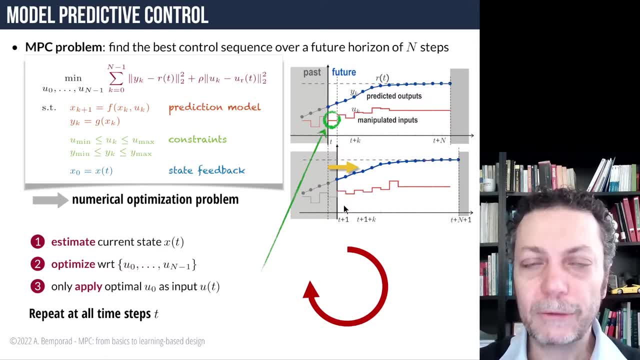 t plus n plus 1, and solve again the optimal control problem, now from the current state x, at time t plus 1.. So in this way, MPC transforms an open loop control policy into a closed loop state feedback policy thanks to this mechanism, which is called receiving horizon control, due to the fact that the prediction horizon recedes over time as we move on. 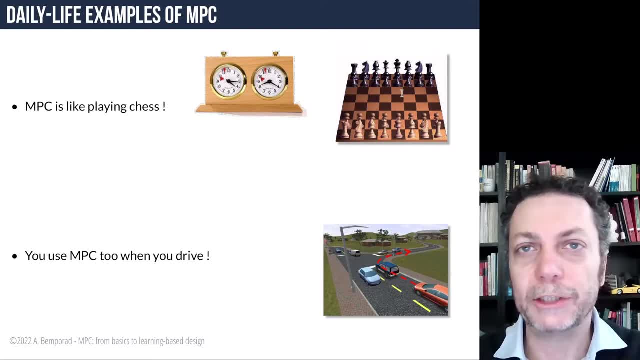 Now, this concept is not new. it's not actually anything strange. This is what we also apply in some daily life examples. For example, if you play chess and it's your turn, what you do is to look at the position of the pieces on the chessboard, which is the current state, and 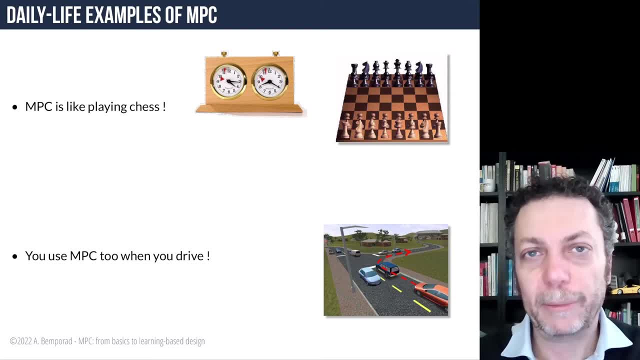 make a prediction of a sequence of moves that you can apply in the future, based on the model of the system, in this case, the way the pieces can move, The various pieces can move on the chessboard- and based also on a model of the opponent and 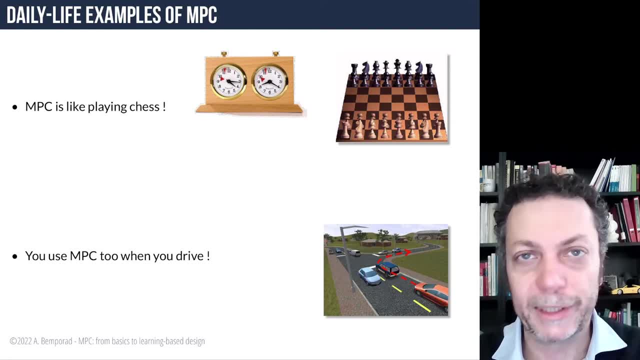 the prediction horizon here depends on how good you are playing chess. The longer the prediction horizon, the better player you are. but when is your turn? you can only apply one move. You cannot apply the whole sequence. You apply your move, the opponent will play and then at the next turn you will. what you will do is to. 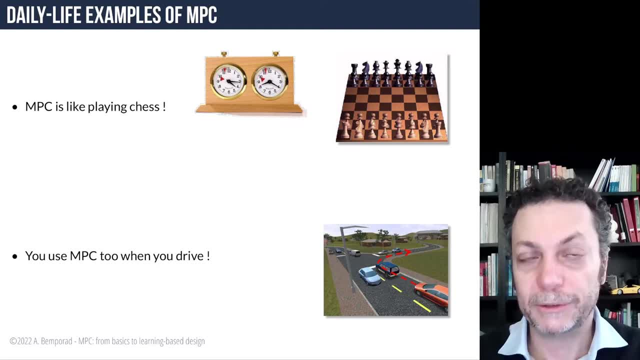 look at the new position of the pieces on the chessboard, Which is your state Xt plus one, and maybe either continue on the same optimal sequence you had before or maybe change the sequence because the opponent has done something different from what you had expected, And similarly when you drive your car. 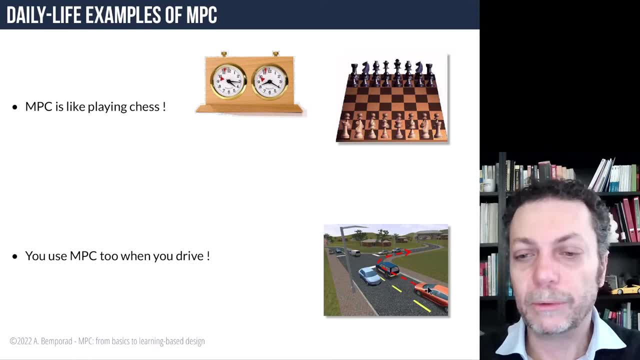 say: you want to go from here- your car is the orange one- you want to go from here to your home, which is some kilometers away. What you do is not to look ahead the entire path to your home, but just look ahead a certain distance. For example, here the distance. 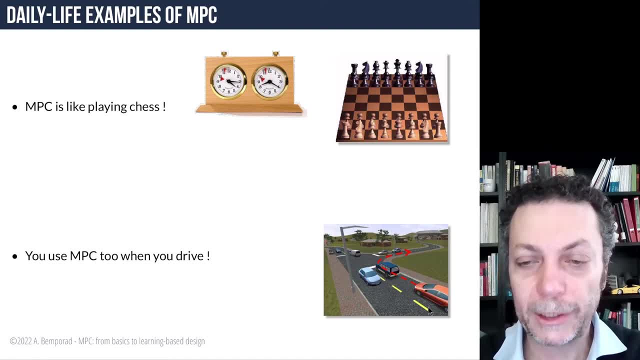 it takes to make the right turn. Then optimize over this short path your sequence of moves, So your sequence of deceleration, acceleration and steering, and then apply the commands. And then, as you move, you will revise your policy. For example, the car in front of you had a different. 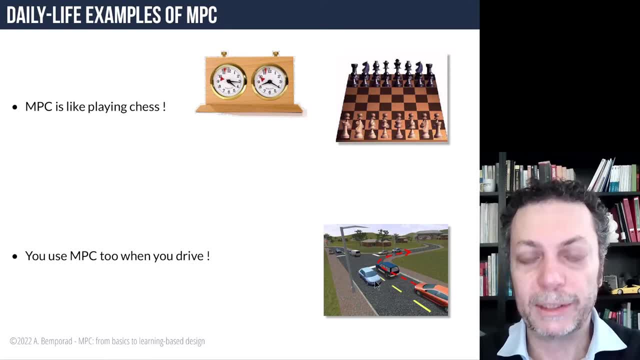 velocity than you had expected, So you have to brake more than you had expected, and so on. And as you move, as you, for example, have turned, then you will look, you will continue looking ahead, further and further over the road, in this receding 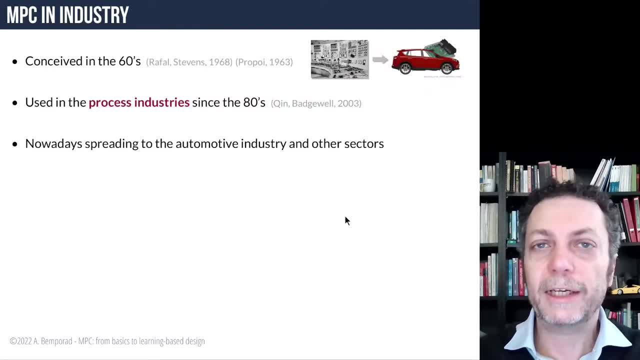 horizon mechanism. Now the idea is also not new in the industry and also in the scientific literature. MPC was conceived around the 60s. First papers that you can track are one by Rafal and Stevens in 68 in the process control community and there is also a paper by Propoi in the Russian literature. 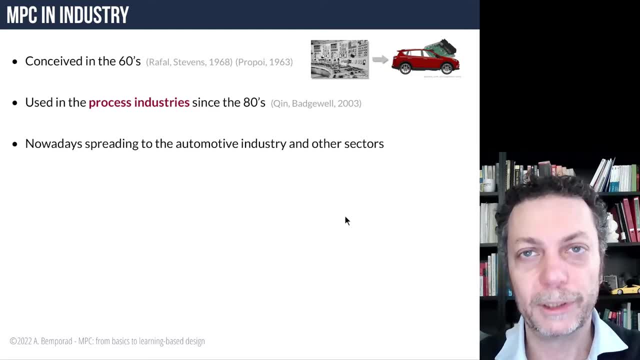 from 63 who proposes the use of linear programming for receding horizon control. and, as a matter of fact, MPC is used in the process industries since the 80s. There are thousands of applications reported of MPC in various various sectors of the process control industry and also other sectors, And actually MPC 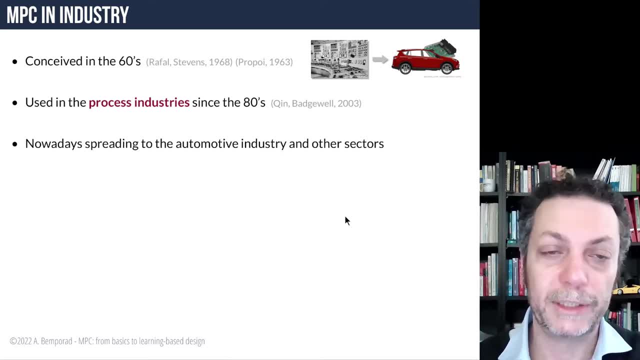 nowadays is spreading a lot in the automotive industry and as well as in other sectors, because of its ability to handle constraints and to coordinate multiple inputs to achieve optimal closed-loop performance. And let me mention one concrete example that was developed by General Motors and our spin-off company, 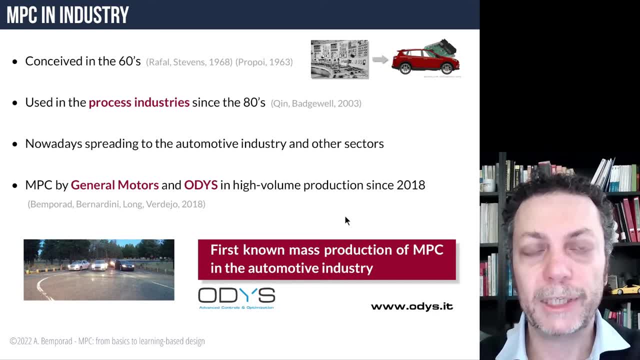 Odis, who designed an MPC controller for controlling the torque generated by a gasoline engine, which is now in high volume production since 2018, late 2018.. And, as far as we know, this is the first mass production of MPC in the automotive industry where the controller runs and 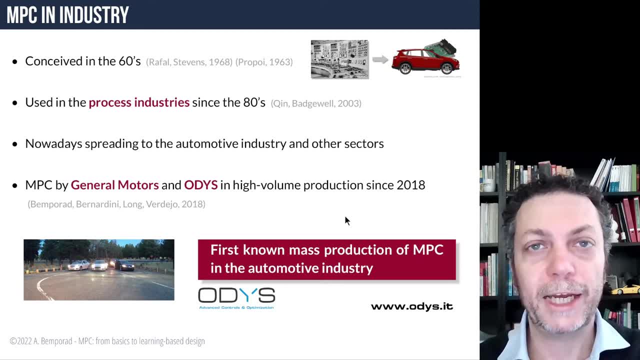 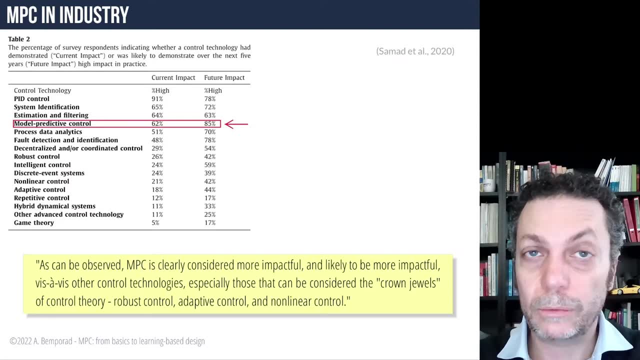 solves the optimal control problem I was mentioning before, in real time on the electronic control board of the commercial vehicle. So to understand the impact of MPC in industry, there have been some surveys run over the years. This is one of the latest, coordinated by Tariq Samad, As you can see: PID control. 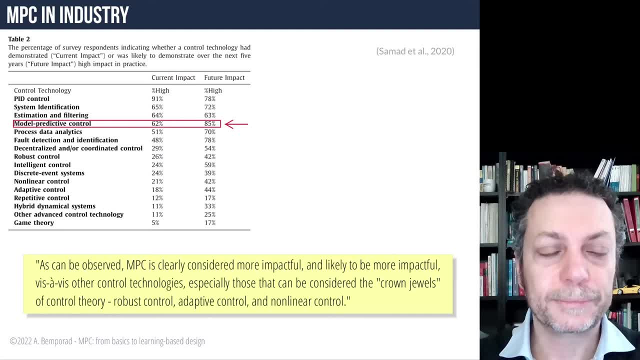 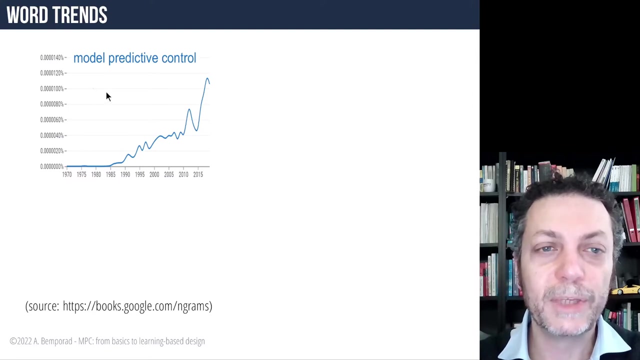 still dominating- and system identification for data-driven control, estimation and filtering. Then MPC comes in as a very impactful and promising which has the higher future impact expectation compared to the others, And I will just base on Google and grams of words appearing in books. If you look at the MPC, what is the trend? 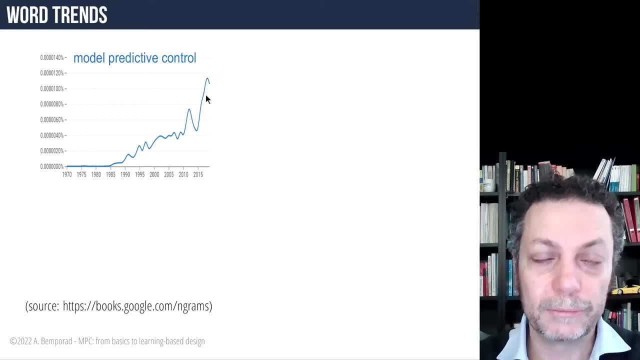 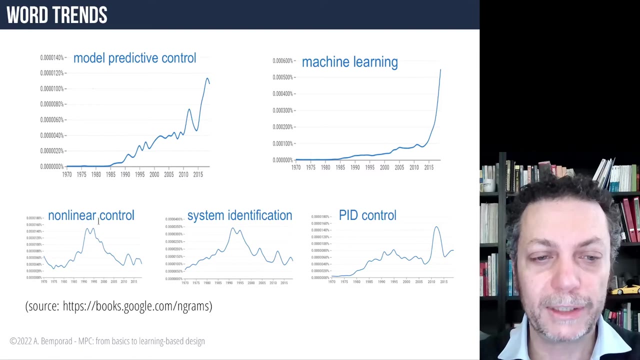 Over the years there is quite high rates of appearances of the word MPC. You can look at machine learning- while other control techniques- linear control- has been had some gain in popularities in the 90s. Then it's kind of stable system: identification, PID control. 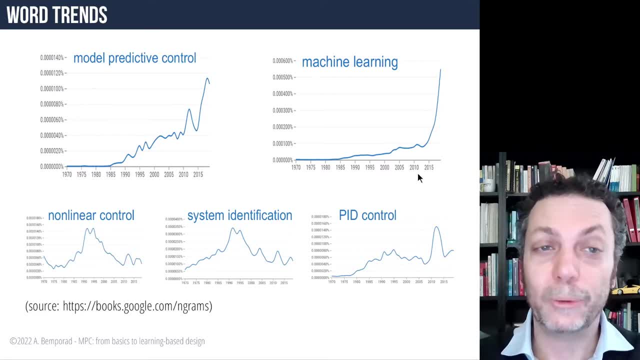 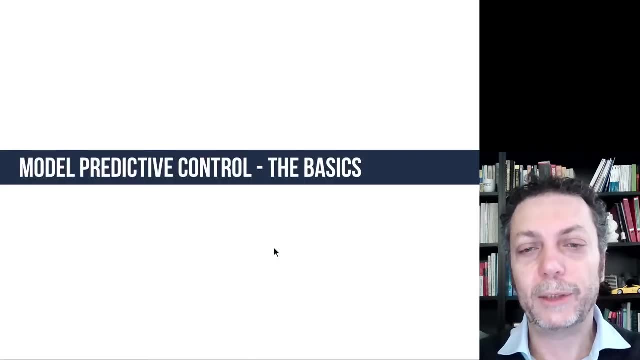 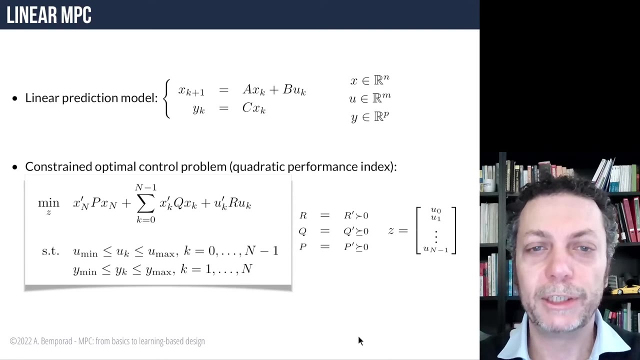 and so on. So this is why today's lecture is on a combination of model predictive control and machine machine learning. So let's start with the, with the basics of MPC. Let's start with the simplest formulation, which is based on linear prediction model. 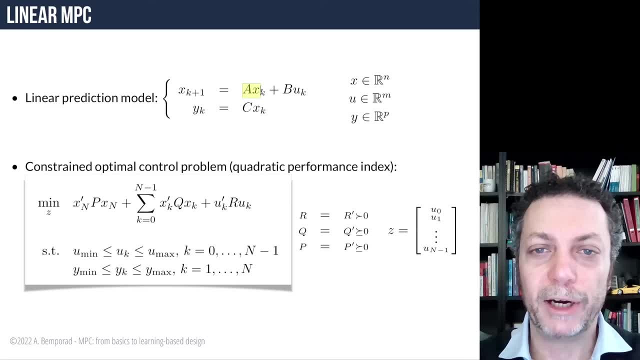 So your system dynamics is described by linear time. invariant system described by some method is ABC. The system in general can be multi input, multi output and let's say we want to control the state of the system to the origin subject to constraints on input and outputs. So here we have some penalties on the states in the form of quadratic forms. 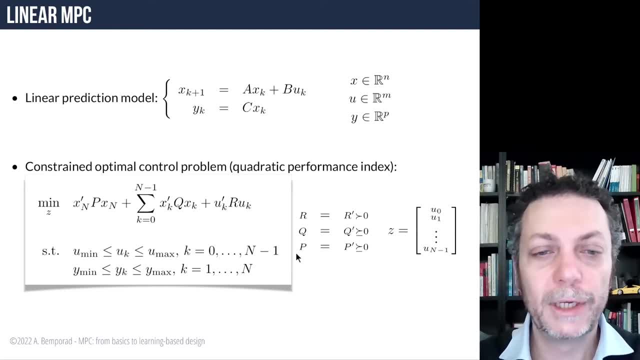 given by some positive, semi-definite matrix Q and also penalties on the inputs, So similar to LQR control, if you are familiar with it. Plus we may have a terminal penalty, So a penalty on the state and the end of the prediction. Now the problem depends on the sequence of moves that I call here vector z, which collects the move. 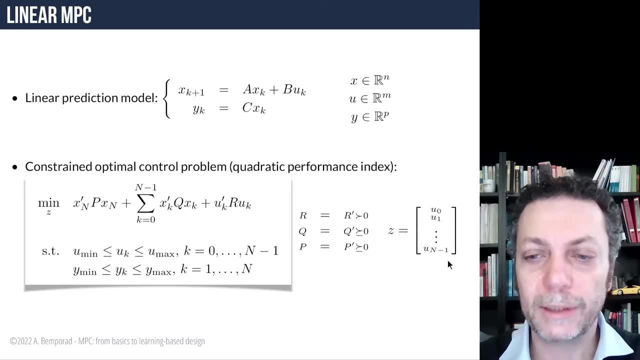 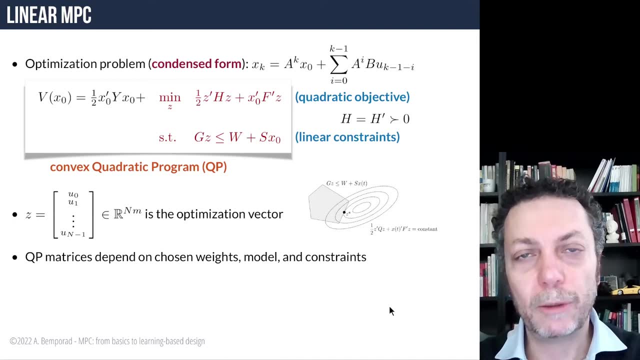 from the current time, u0, u1 up to ul-1 at the end of the prediction. Now you can show easily that you can map this optimal control problem into a quadratic programming problem. So the function that you are optimizing here can be expressed as a quadratic function of the vector z. 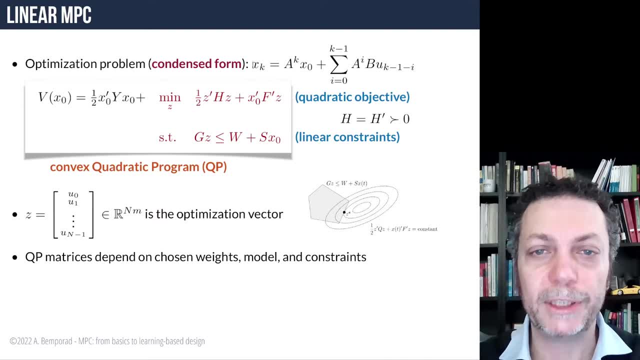 of moves, for example by substituting the states during the prediction as a linear function of the initial state, and the applied inputs, and, as well as the constraints on inputs and outputs, map into linear constraints on the sequence of inputs. Okay, this is a quadratic programming problem that, if you know how to solve it, will give you an optimal sequence of moves. a vector z of control moves. 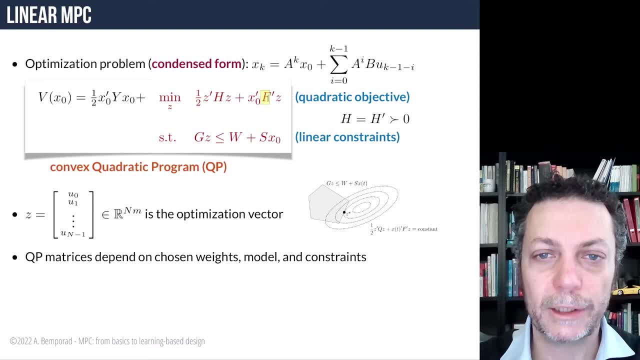 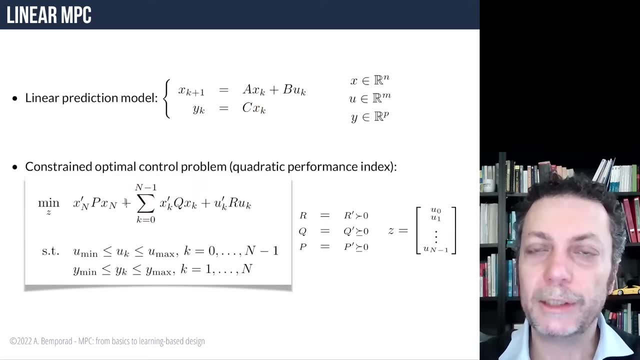 and, of course, the QP matrixes that you see here- h, f, as well as the constraint matrixes g, w and s- depend on the weights that you have chosen in the control formulation, as well as on the upper- lower bounds on the inputs and outputs. 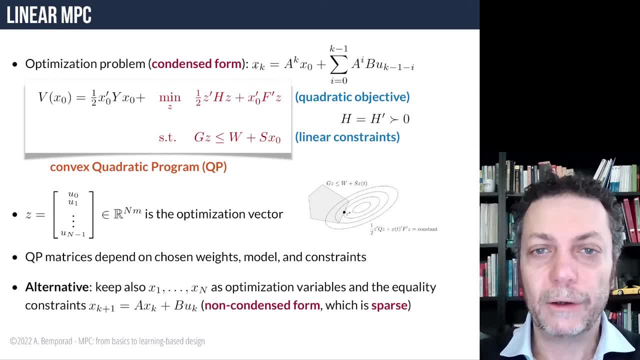 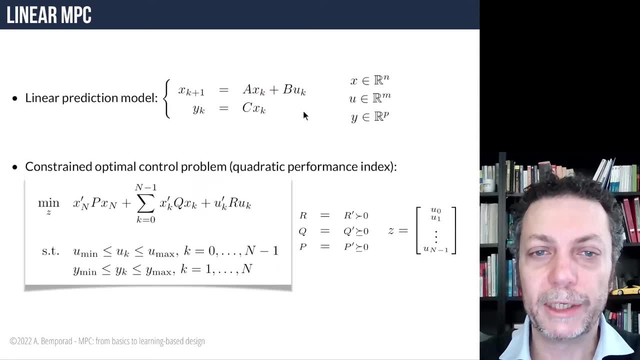 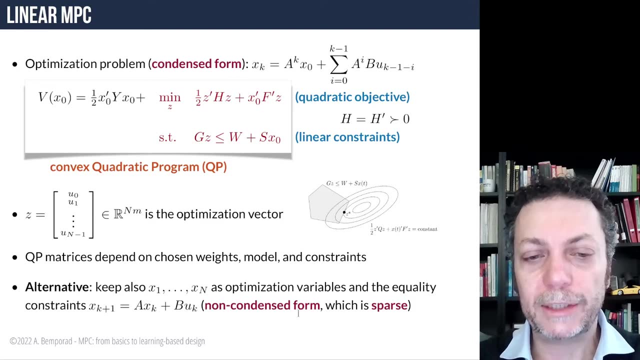 So this is called actually the condensed form, because you got rid of states by substituting states, So by removing the equality constraints due to the system dynamics, you can also use an alternative and non condensed form where you keep such linear equalities and optimize with respect to both inputs and states. And this is, you have a larger number of variables, but the problem matrices have some more. 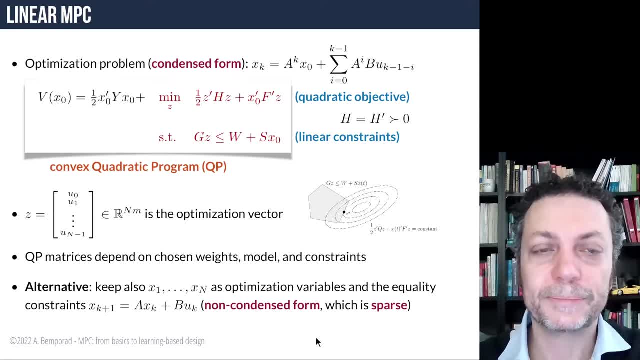 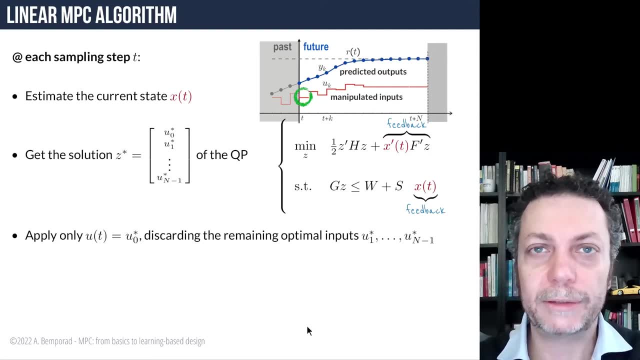 structure that you can exploit, that some solvers exploit. So the linear MPC algorithm, then, will work like this, according to the receding horizon strategy that we have introduced before: get the current state or estimate it by means of an observer, solve the quadratic programming problem, take the solution and only apply the first move of the solution. 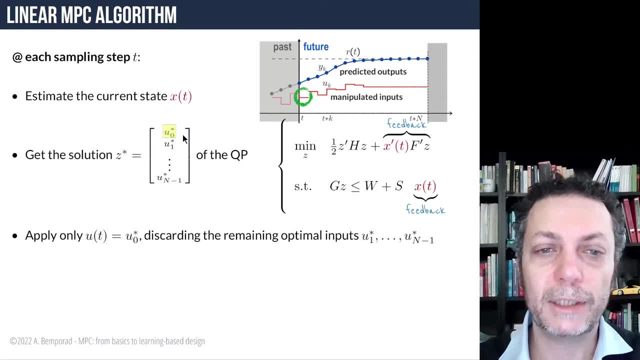 So the first entry in the in the vector, so the all the entries related to the input at time, u t plus zero, and apply this to the system. And you see here why is the state feedback? because the state appears in general in the right hand side of the constraints. 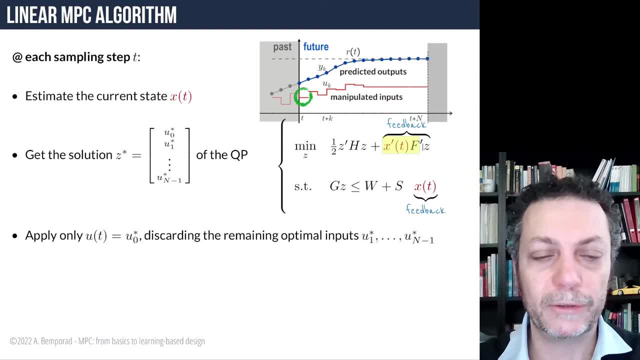 If you have state related constraints and in the linear term of the cost function. and of course, you discard the remaining samples because you're not going to apply them, because the next time step t plus one, you will do the same with the new state Xt plus one. 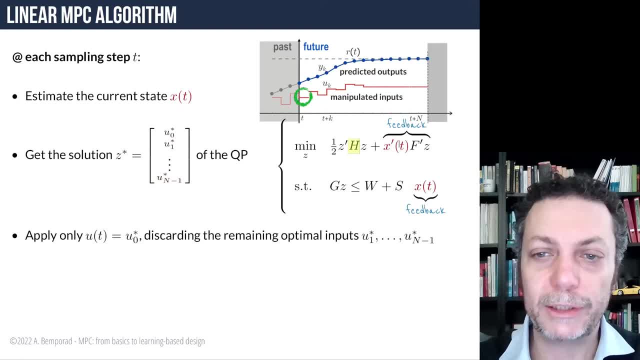 and then Xt plus two and so on, and note that the matrixes here don't change. So in case we're using a linear time invariant model and the cost function and the constraint don't change- H, F, G, W and S, these are all matrices that you can compute beforehand and store. 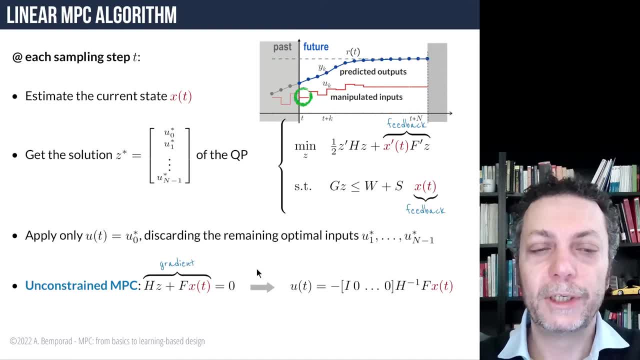 now what happens in the case of unconstrained NPCs. so let's say you don't have constraints. then the problem is much simpler because you have a closed-form solution. your function is a quadratic function of Z, which is has a minimum when the gradient of the function is equal to zero. here the 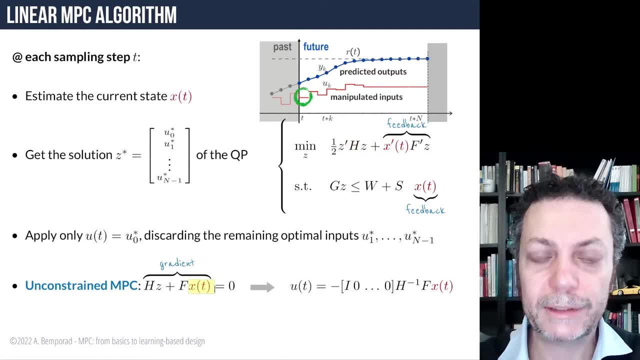 gradient is H, Z plus F, X, which is zero. if Z is equal to minus H, minus one F time X of T. and since you are extracting the first component, just multiply by a matrix I, and then zero, zero, zero, the identity, and then zero, zero, zero to. 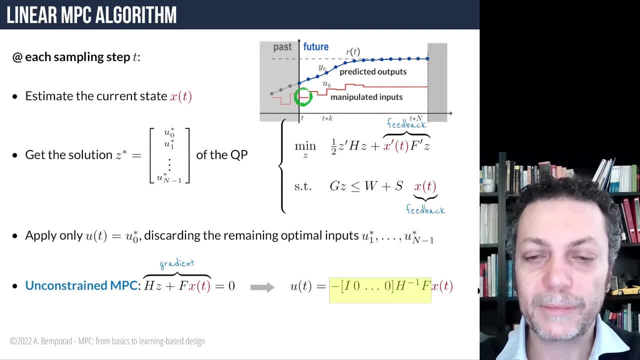 extract the first input and what you have here. this is a constant time function and you can compute the cost function and the constraint. don't change matrix or row vector. if you have just one input, which you can call K, it's a constant state feedback. so NPC without constraint, based on linear model, is 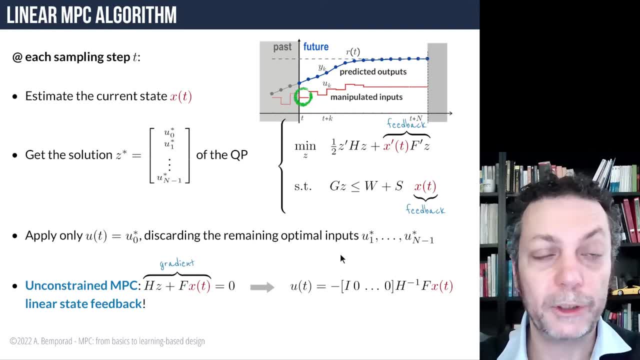 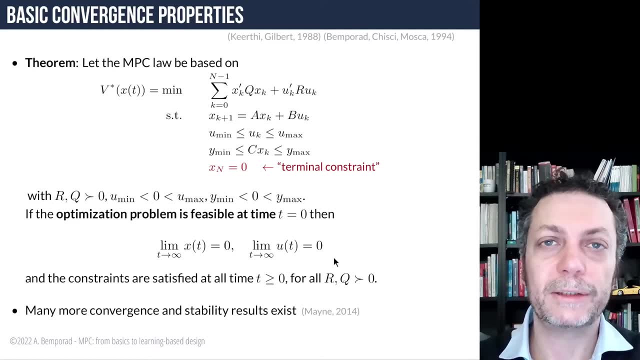 nothing else than a linear state feedback controller, you can prove convergence and stability properties of NPC. there is a rich literature on this: this nice paper by Main 2014 that surveys a lot of the best techniques that were available that time for proving closed-loop properties of NPC controllers. of course, the field has 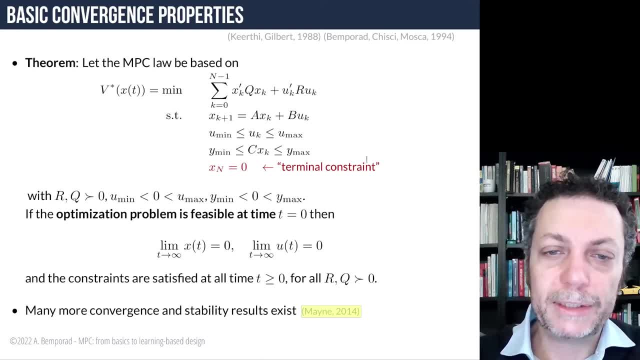 evolved since then. here is a is a result that it's actually one of the simplest you can. you can tell about the NPC. it's about convergence of the scheme that I have stated just now, where, in addition, I'm adding a terminal constraint on the state at the 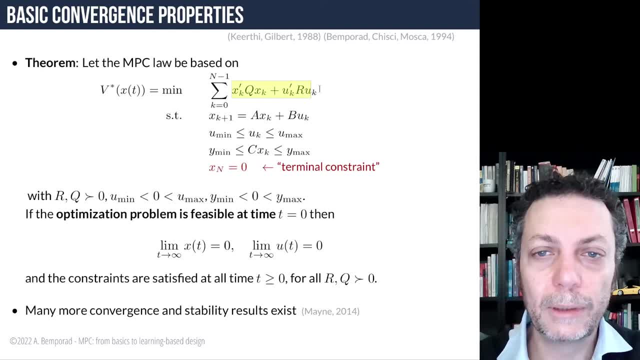 end of the prediction. so if you minimize the quadratic cost shall be subject to the linear dynamics, possibly linear constraints on the inputs and the outputs, and you also impose a constraint on terminal state. you can show that for any choice of the weight matrices Q and R, they are 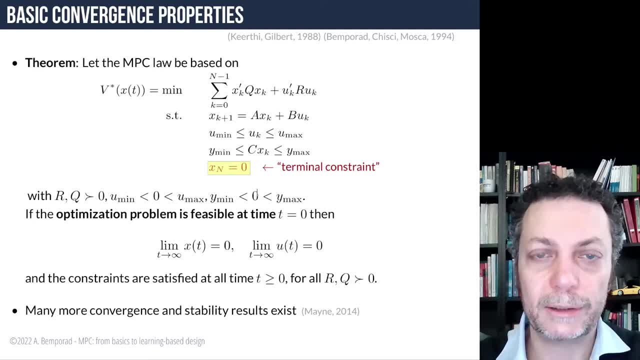 positive definite and if the zero is is an admissible value for the upper lower bound is strictly inside the range of admissible inputs and outputs, then you can prove the following: if the problem is feasible at time zero, then you can show that it will be feasible at any time step and then the state will. 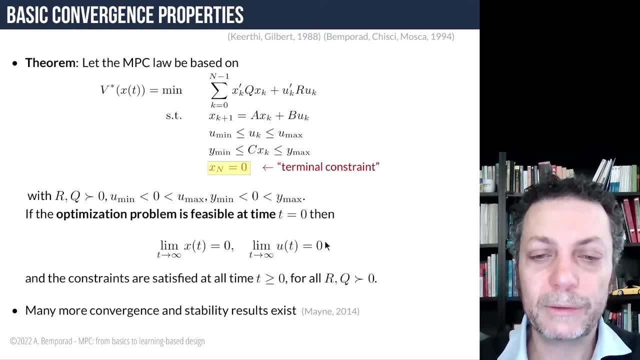 converge the origin. the inputs also will converge to zero and the constraints that you have imposed will be satisfied at all time t greater than zero. okay, this is just a basic result, the proof. we're not showing the proof here. it's based on showing that the optimum that you get by 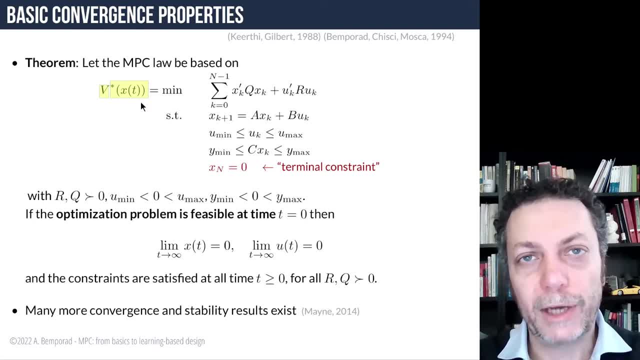 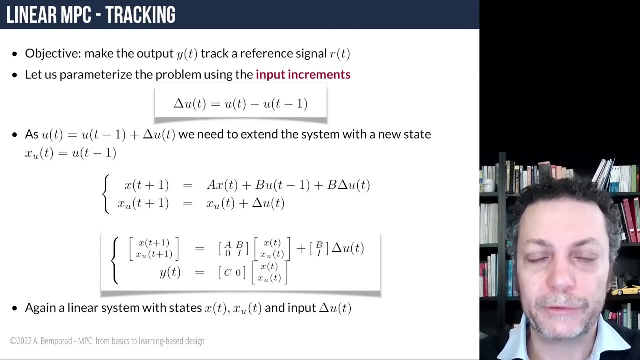 solving the problem behaves as a Lyapunov function for the closed-loop system, so you can show that this decreases over time and, from this, show that the actual trajectory needs to converge. okay, now what if you want to track a reference signal? so so far we have seen state regulation. now let's see what. 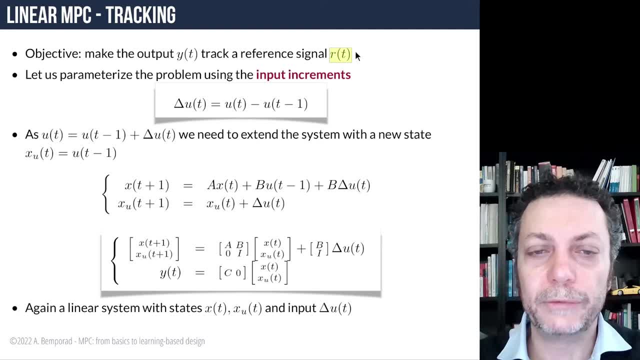 happens if you want to track a certain reference R. well, one approach is to formulate the problem using input increments. so let's call delta u the difference between the current inputs and the previous one. you can describe the dynamics now with an additional state which is the integral of the input. 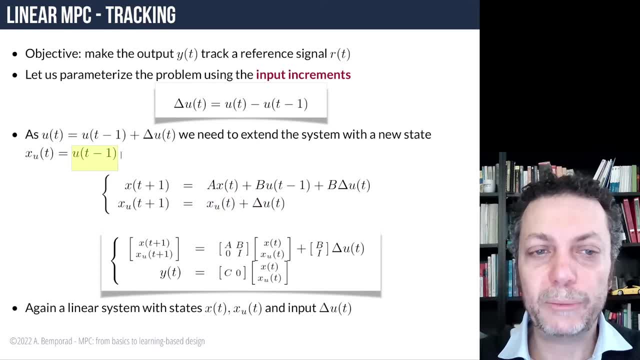 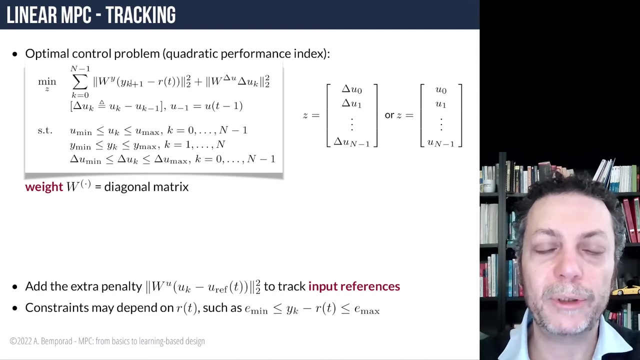 increments. so let's call X, u the previous input, so that u of t becomes the previous input plus the increment. so by extending the dynamics with the previous input at the state you can look at the extended system and directly optimize over the delta u's. so if you now set up a problem, where now 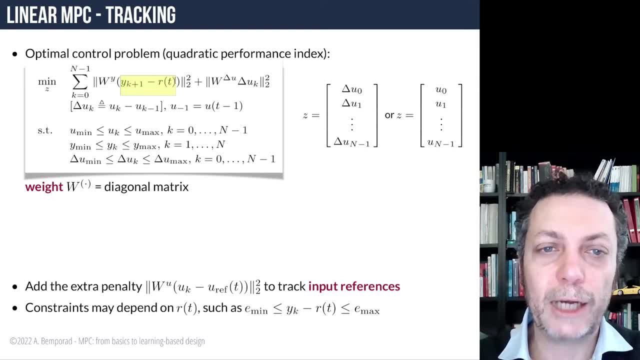 you penalize the difference between the predicted output and the reference and the penalty you are the penalty on the input increments. so the idea is that this cause is zero if you're doing perfect tracking, because the tracking error will be zero and at steady state. if you're tracking the 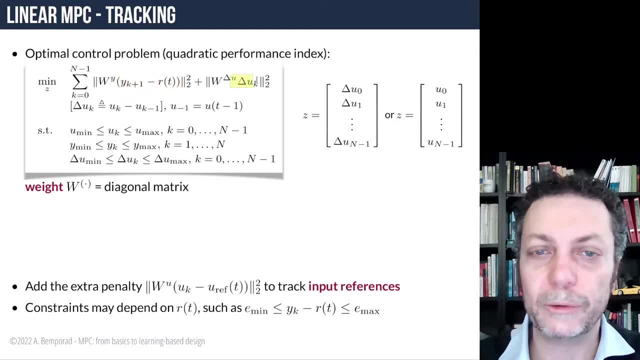 reference signal R of t, the input will be constant, so the delta u will be zero. if you're optimizing, this problem is subject to constraints- gain on input and output- and this point also constraints delta u if you want to include to take into account zero rate constraints you may have on the actuators and 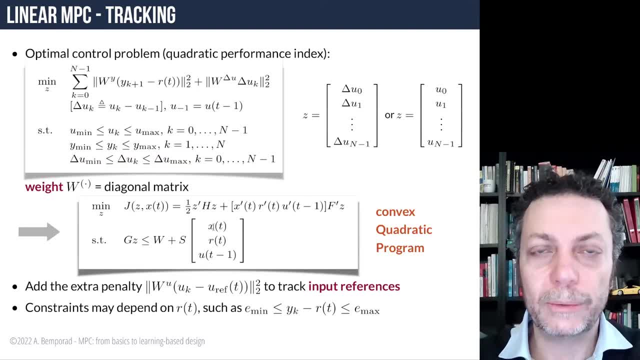 regist körte. these Fen ci g, pro audit parameterize, the pro office backed input, the sickness of inputs. now this reference and the previous input appear in the right hand side. all the constraint аго on the integrated stage linear term of the cause function. now what are w, y, w, delta, u? this could be diagonal matrices. 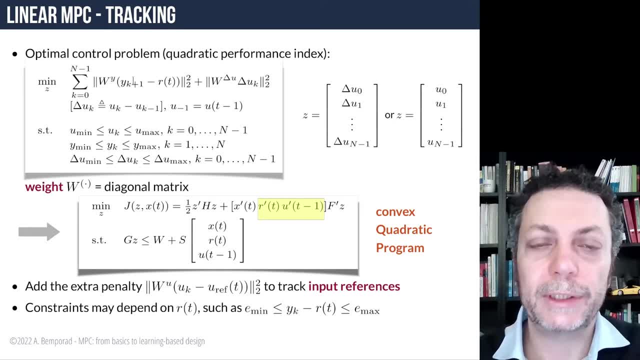 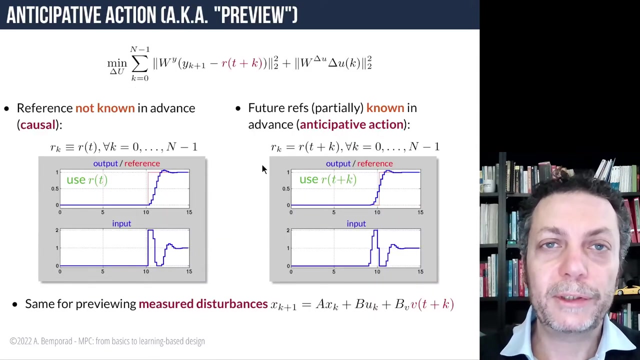 so to weight tracking error, different tracking errors and different input increments differently. you may also want to add: if you have an input reference in the cause function weighted by some other weights- w, w- okay, so this: this can be a formulation for tracking and this works well in practice. you can even include preview on the reference signal if you have knowledge of future. 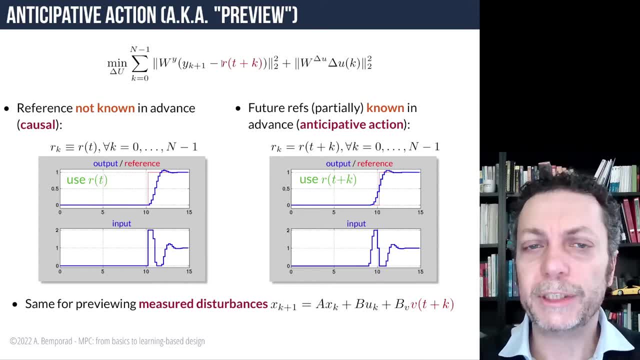 references in advance, which is not so a weird assumption. for example, in repetitive tasks you know the reference in advance or the reference may come from another optimization. so you have two layers: optimization, where the higher level optimize the sequence of references and this is passed to a lower level, handled by our npc controller which consumes this. 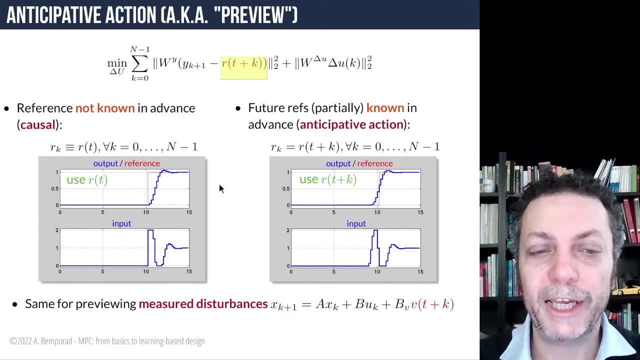 sequence of references. and here you can see how the controller behaves if you have no information about future reference. so the system is completely causal. it only knows r of t, doesn't know the future once. and you see here an example of a step response. the system will respond after the set point change happens, while if you know the reference in advance, 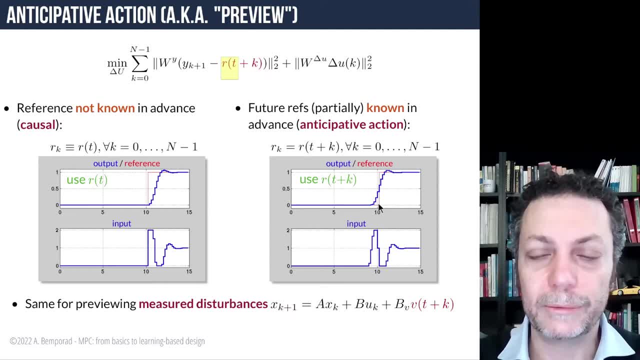 you can achieve this anticipative action. it's a non-causal control action that naturally pops up. and also you can do the same preview if you have the measure disturbances. so you can extend the model with major disturbances. if you have signals that you can measure and you know, enter the model. 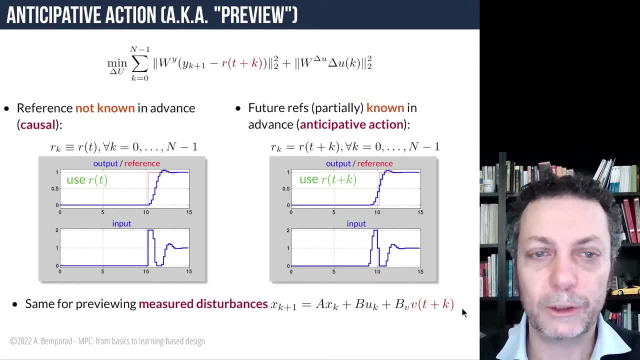 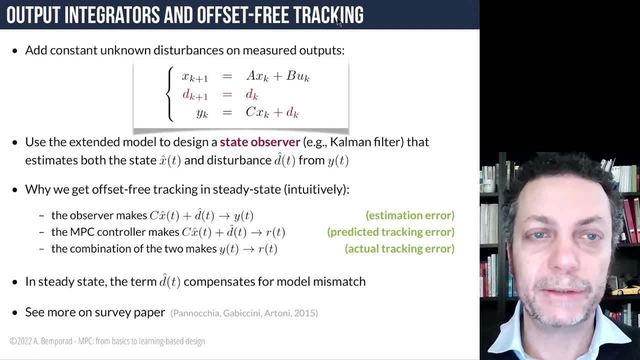 and also keep this preview information into account in the optimization. there are a few ways of making sure that npc achieves zero tracking error in steady state. one popular one that works really well in practice is to introduce output integrators in the model and use them in a state. 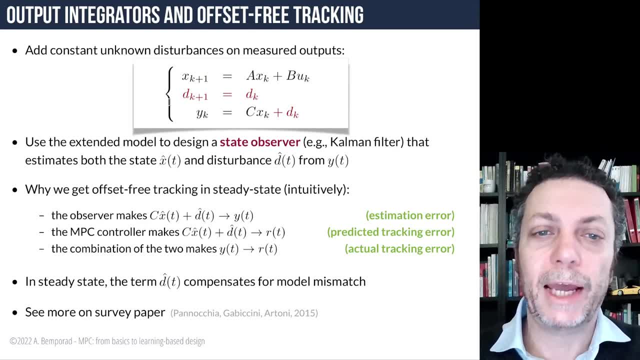 observer. so the idea is the following: take the model and add a constant state, which represents a disturbance that acts on the output, and it is the value that explains the difference that you have between the output predicted by the model and the actual output that you are measuring from. 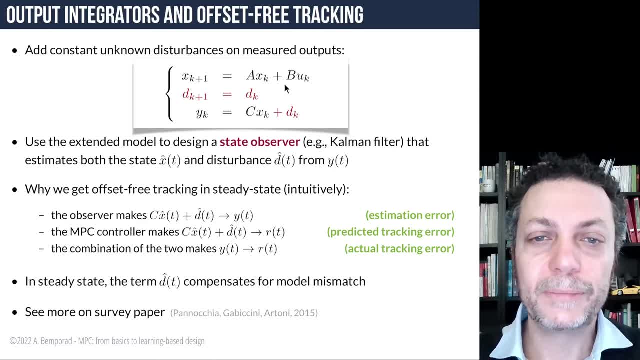 the system that you want to track the set point. so with this model there are different forms of disturbance model you can use. you can look at this paper by panokia and others which is a good survey on the topic. then, with the state observer, if you provide the npc controller, 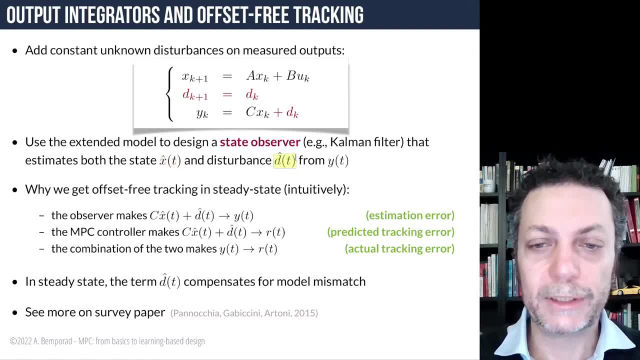 the estimate of the state and together with the estimate of the disturbance, then what happens intuitively is that the observer will try to reduce the output estimation error, so the difference between the output predicted by the estimate and the measured output, while what the controller does, taking the value of the state, will try to make the predicted output. 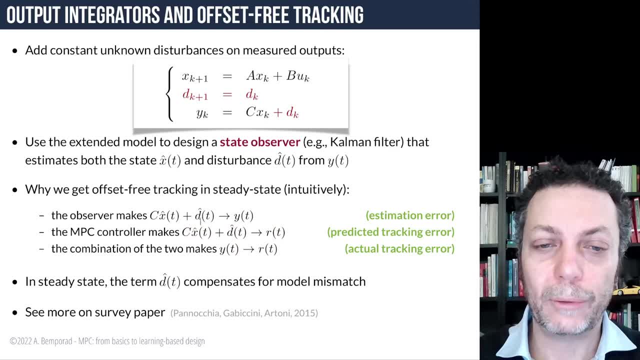 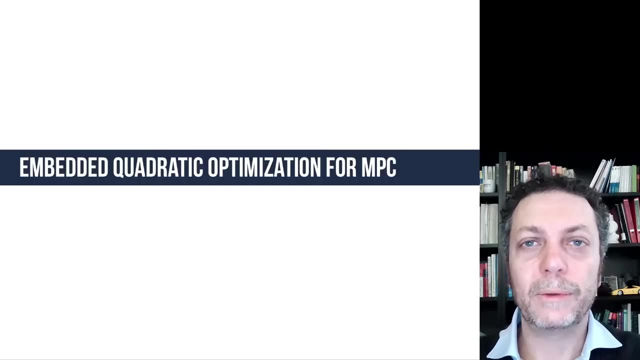 track the reference signal and, as a result, if you combine these two, you have that y of t will track the reference signal. okay, so this is not a formal proof, but it's a an explanation why these schemes work well. okay, now we want to address the problem of solving the npc problem and, in particular, we 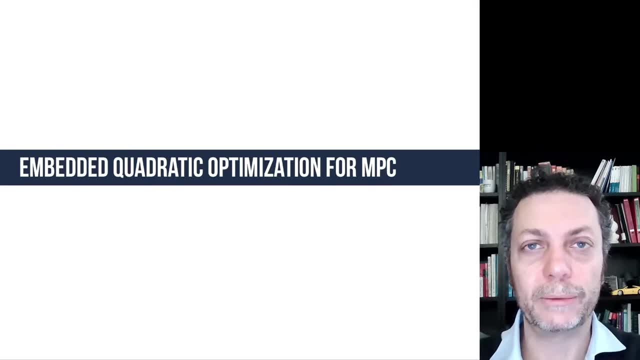 have seen so far formulations of the optimal control problem we need to solve as a quadratic programming problem. so what i want to spend time on now is to review a few simple quadratic programming problems that can be used for online optimization. so let's restate the problem: minimize the quadratic. 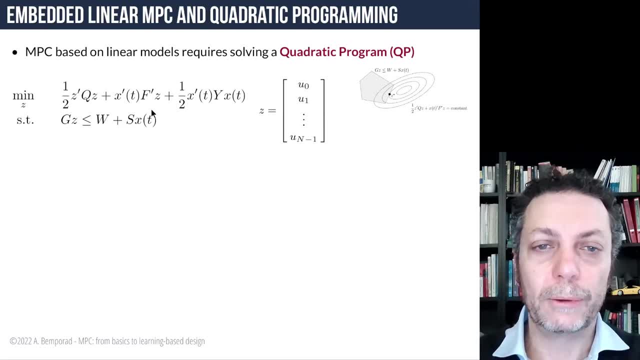 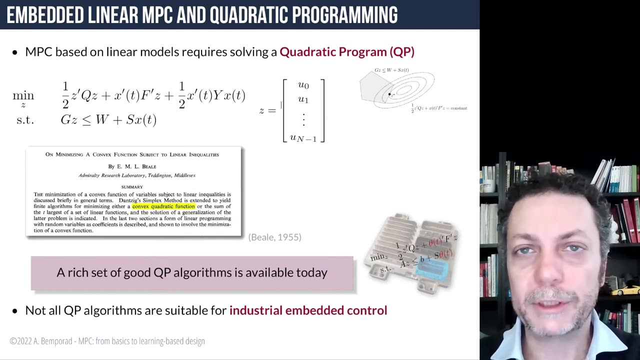 function. that comes from the optimal control problem and let's use the sequence of inputs as the vector that we want to optimize. now. solving a quadratic programming problem is not a new problem. one of the first papers presenting a solver for such a type of mathematical programming problems- the paper that dates back to the 50s. i build so since then. 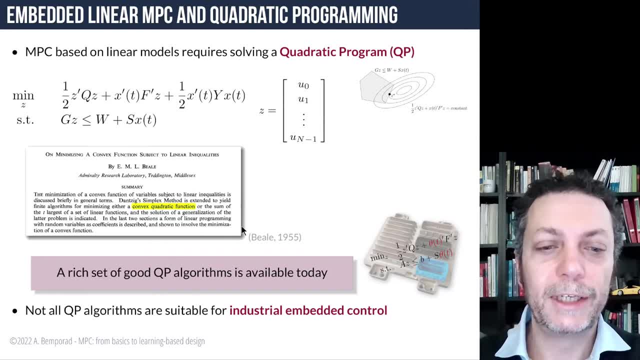 in the last, say, almost 70 years, there have been a lot of good ideas on how to solve qp problems, so as a result, there is a rich variety of solvers available for solving this type of quadratic optimization problems. of course, not all the algorithms are good for embedded control, so not all algorithms are amenable for being implemented on a. on a. 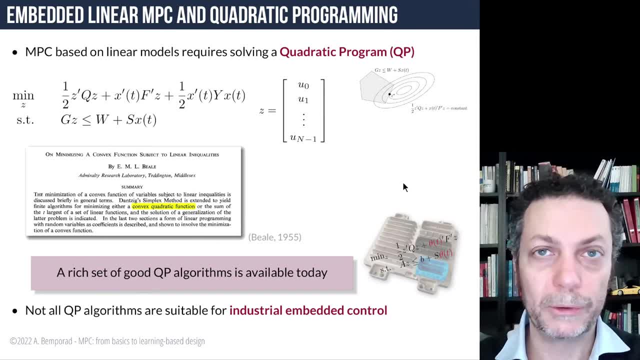 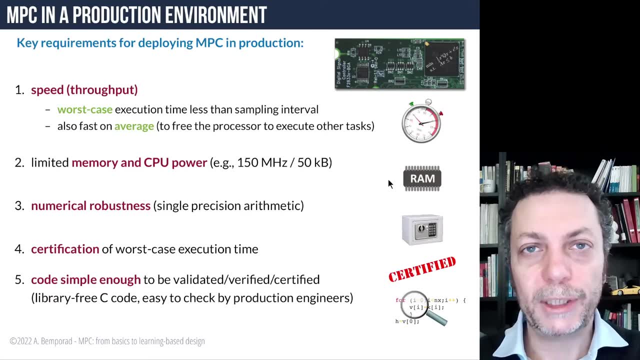 control board, for example on an electronic control module of a vehicle or a microprocessor. so let's see what are the requirements that the qp solver must must enjoy in order to be a good candidate for deployment in a production system. of course, speed is a requirement, so 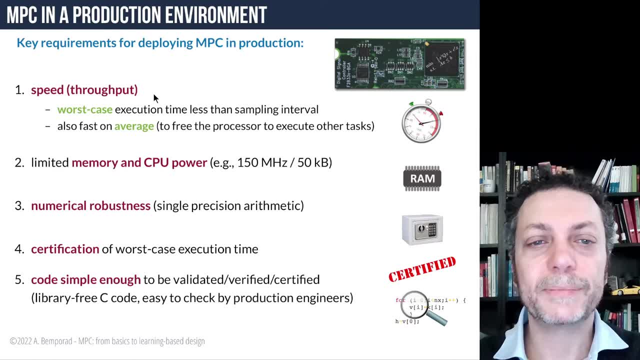 must deliver solutions in a in a short time, especially in fast sampling applications, not only on average. so what is important in the npc is not only the average time it takes to compute the solution, but also, in particular, the worst case time, because you want to make sure. 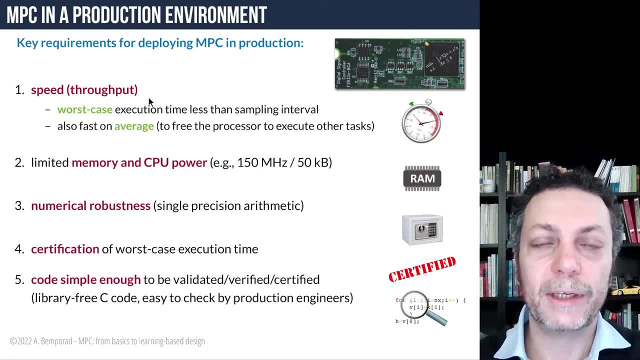 that at every sample step you are able to provide a solution to the problem, which means to provide an actuation signal to the system. it also matters the be. the processor must also solve other tasks. the the load of the process will also depend on the average cpu time required by a solder. 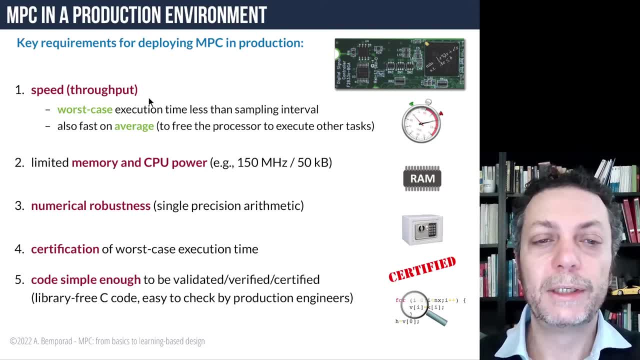 now, another aspect is still very important many applications is memory, and another aspect which is very important is numerical robustness. i think that still many of these algorithms are implemented in single precision arithmetic. this probably will change in the next years, but that's the current situation situation. So you must have an algorithm that is robust with respect to numerical errors. 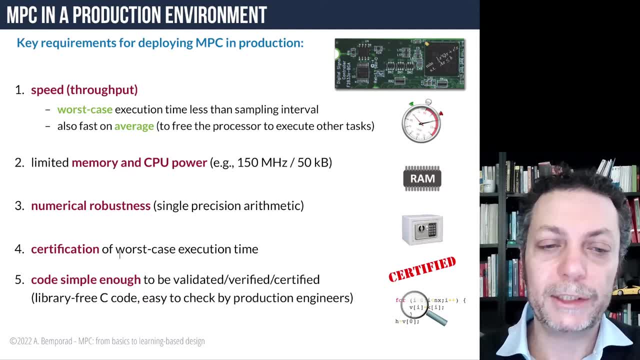 And you must be also able to certify the worst-case execution time. So your piece of software that solved the problem must be able to to be certified for what is the number of flops it makes in the worst case to deliver the solution, And as well as the code that implements the solver must be not too complicated, Otherwise you cannot run. 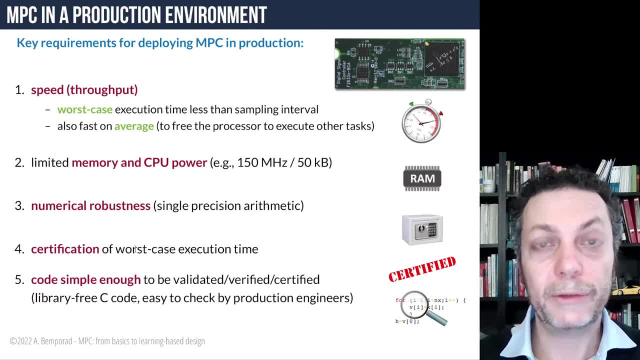 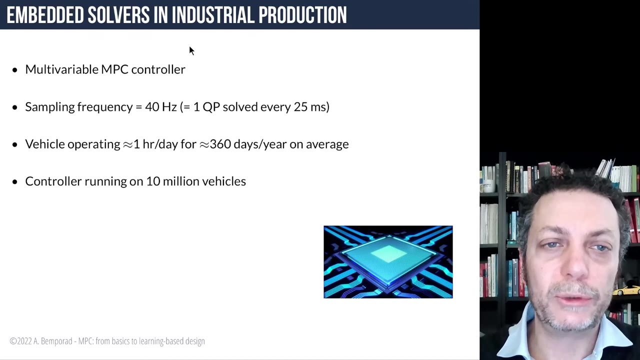 software analysis packages or even formal methods to validate and verify that the control system satisfies the properties you want to satisfy. This is particularly important in safety-critical application. So let's let's consider an example. So let's say you want to design a multivariable controller. 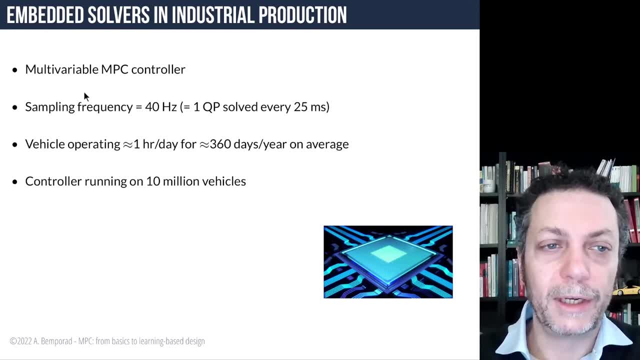 This is actually an example that comes from a real problem. Say you are applying the controller at a frequency of 14 Hertz, which means you need to solve one QP every 25 milliseconds, And say this is running on a vehicle that on average you could say that operates about one hour per day over. 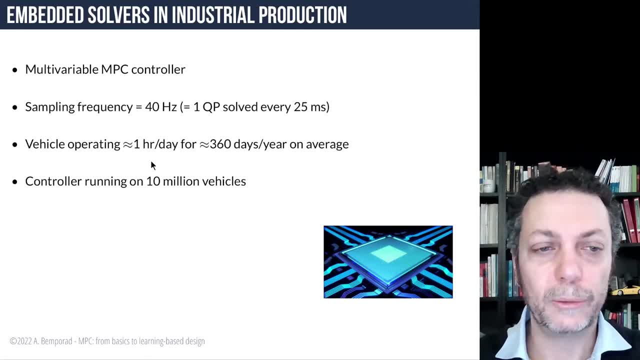 360 days per year, just to make rough computations. and let's say you have 10 million of vehicle in production running this controller. so now, if you do some simple math, you will discover that you are going to solve about half quadrillions of qp problems every year, and then no one of them should should. 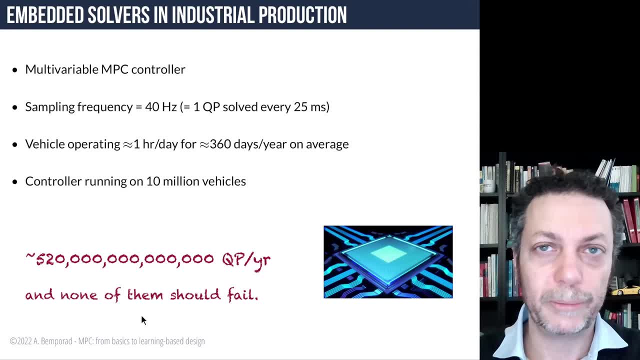 fail. so they must all deliver a solution, otherwise you may have to recall the vehicle or even the whole, the whole flow. you want to do that. so that puts some kind of pressure on on us designing the controllers, because we must be able that the software really achieves this quality. 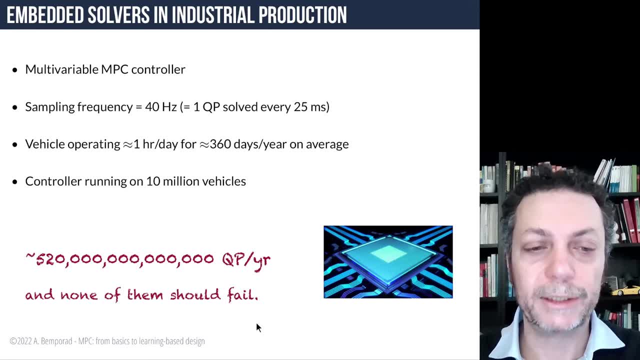 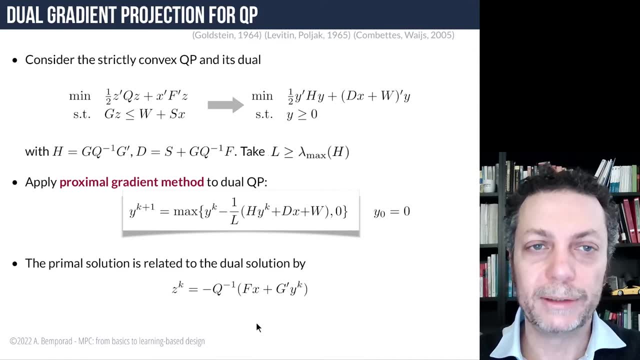 the standards of quality for for reliability. so which are algorithms that are amenable for embedded optimization, in particular for npc? one of the simplest algorithms that you can think of is the gradient projection method. it's an old method that was proposed for convex optimization that you can apply on the dual problem of the qp. so let's consider again the qp problem. 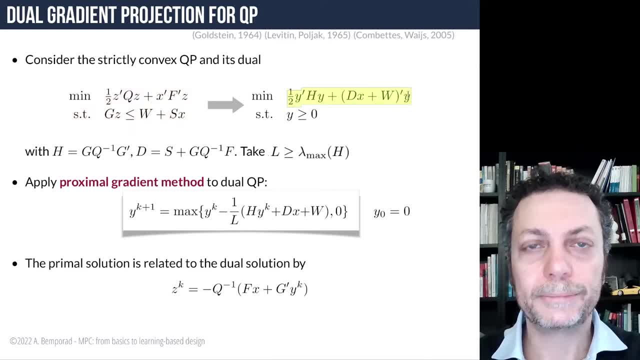 if you form, it's a dual. so the the problem in which the optimization variables are the lagrange multipliers or the regional problem, you can transform one to another. then you can apply the gradient projection method to this dual reformulation, and the reason is that here the projection is simple. 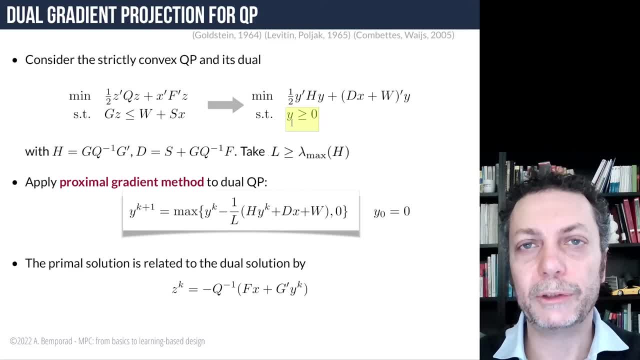 because you just need to take the value of the dual vector and then clip the non-negative, clip the negative components to zero during the iterations, and the dual matrices are constructed from the primal problem by simple algebraic manipulations. now the method is basically one line. if you want one line of matlab code, if you don't include termination criteria, so you start. 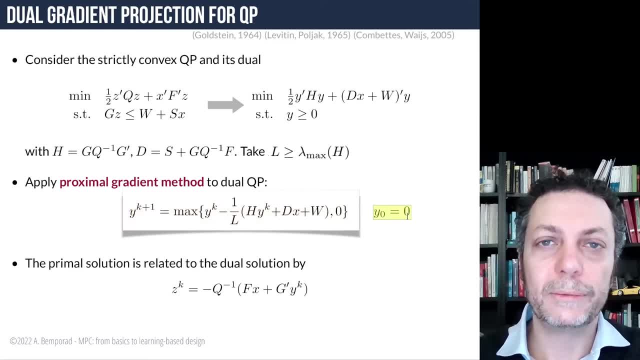 for example, from the zero vector of dual variables, which correspond to the unconstrained solution of the original qp problem, and then make a step into the direction of the gradient of the dual function by some quantity 1 over L, where L is related to the Lipschitz constant of the gradient. 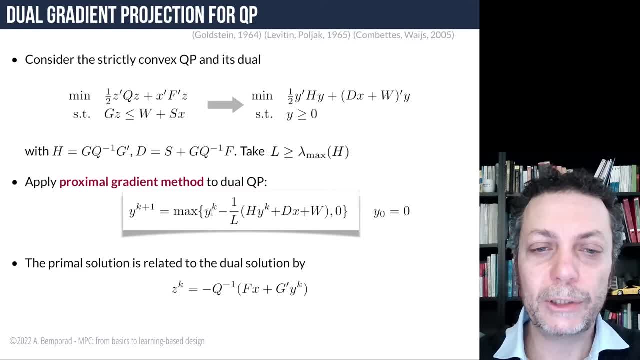 of the cos and then update the gradient to the final function, the dual vector, and project it to be always non-negative. So if you iterate this, you can show that you converge to the optimal solution of the dual problem. so to the dual optimizer from which you can retrieve the primal optimizer of the problem. So very simple. 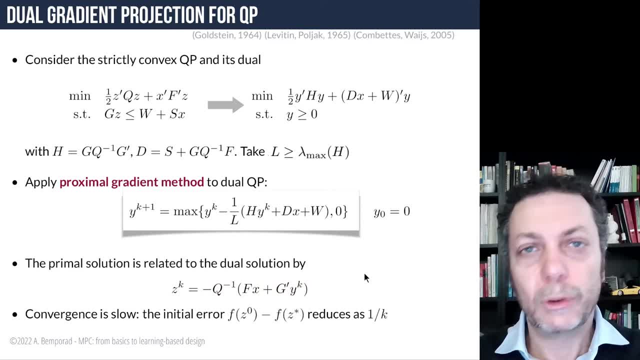 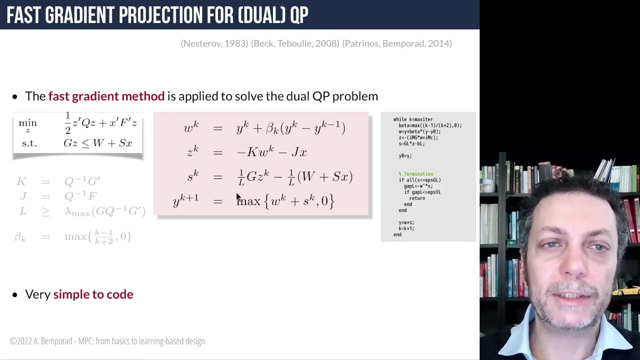 algorithm to code. Convergence speed is not so great. You converge, but the difference between the value of the function at the initial guess and the optimum reduces as 1 over k. Now a better method is the fast gradient method applied to the dual problem. So you can take Nesterov's. 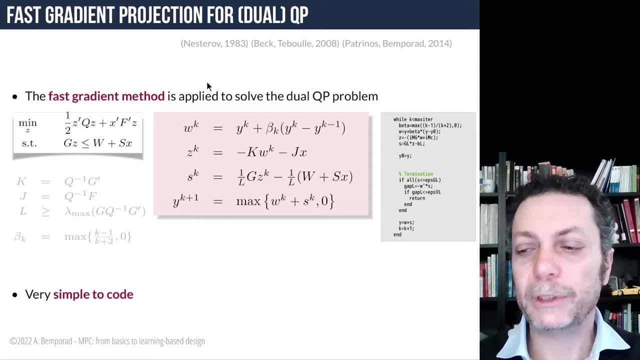 fast gradient projection method and apply it to the dual of the QP problem we have just seen. We have described this in a paper with Panos and Patrinos some years ago. You can rearrange the algebraic operation of the solver into an update of a vector w and 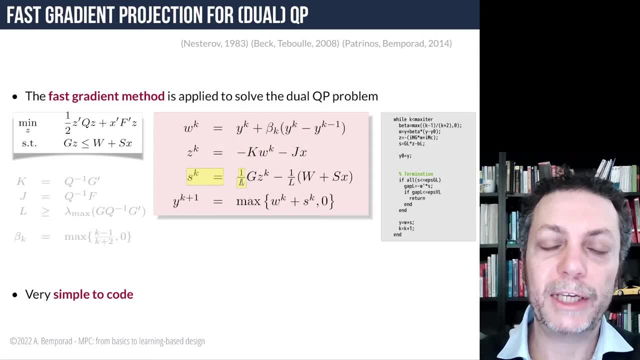 an update of the primal vector z and an update of a scaled version by L of how much you are, you are violating the inequality constraints. And then the projection step. Okay, so if you iterate this, which, in embedded math, is a few lines of code, 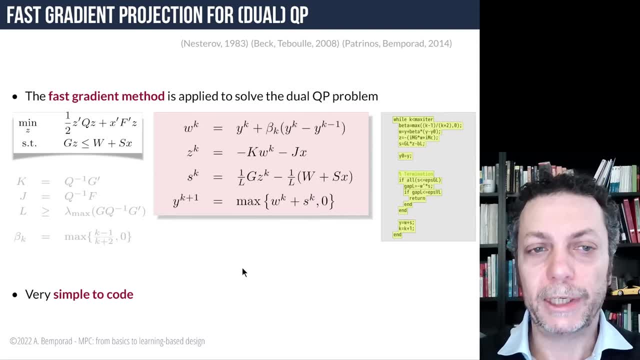 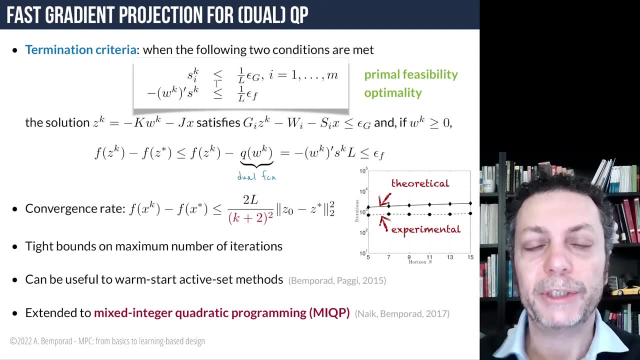 so it's very, very simple algorithm. then you can show again convergence to the solution and you can also derive some termination criteria. So for example, you can stop when you are both feasible by certain tolerance- epsilon, and- and also if the w vector you have is non-negative, you can also estimate the duality gap, So the difference between the 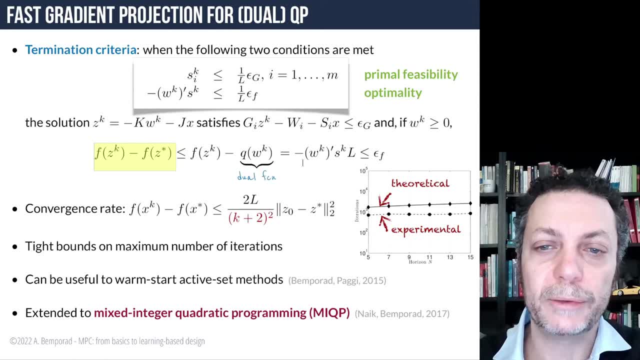 the value of the function at the current iterate and the optimum is upper bounded by this scalar product between wk and sk, and you can decide to stop when also this value is below some certain optimality threshold. epsilon f: In this case, the convergence rate is better than. 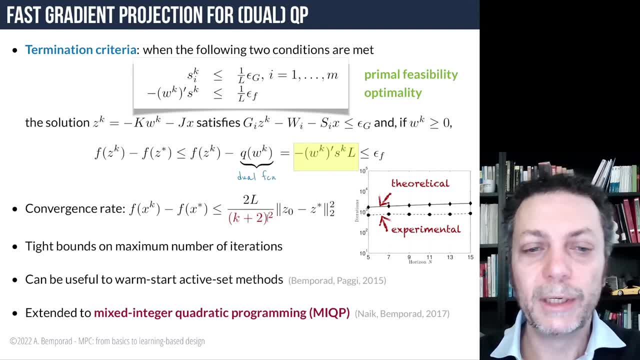 just gradient projection, it goes as a one over k square. You can actually show that also the number of iterations can be bounded as a function of x. So remember in npc x is the current state or current state and reference signal in previous input. 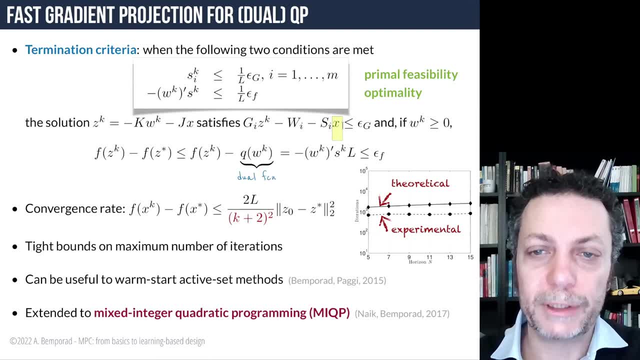 So that you can a priori estimate, for a certain range of x, what you can expect in terms of number iterations and therefore, therefore, number of flops. You can also use this method to get worm starts and then switch to other methods, For example in this paper here. 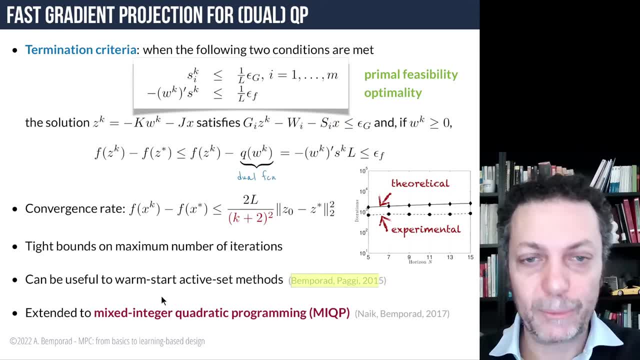 we are shown that you can run a few certain number of fast gradient projection iterations and then switch to an active set method and this speeds up on average the convergence of the problem. And you can also use this solver within a mixed integer quadratic programming solver that you need to 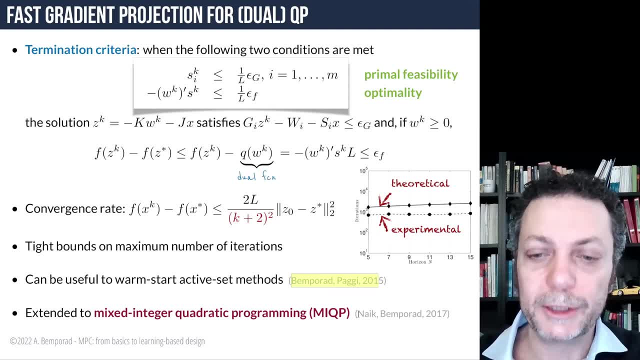 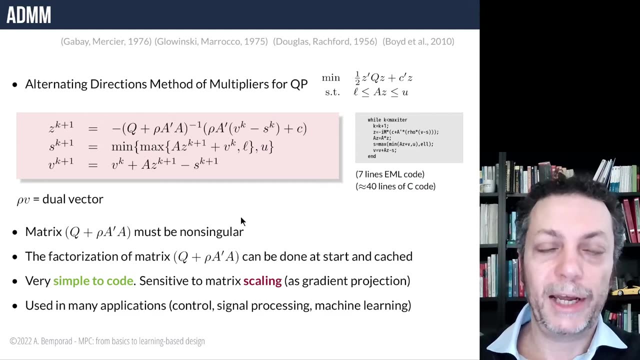 solve hybrid npc problem. We'll see this later And, for example, we have reported some formulations and numerical experiments here in this paper we had made some time ago. Now, a different method that you can apply to solve this type of quadratic programming problems is ADMM, the alternating direction method of multipliers. 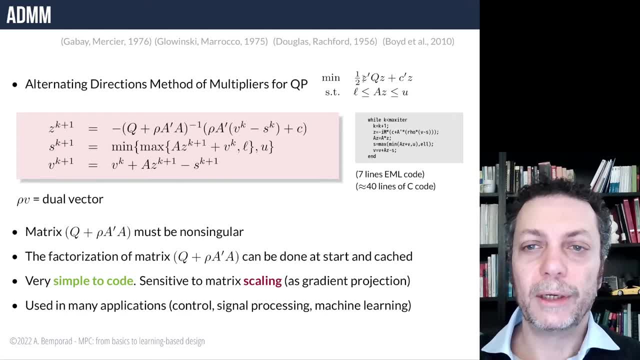 which, in the case of QP problems, where we have quadratic cost and we have linear inequality constraints, In general, we can formulate the constraint as bilateral inequality constraints and even equality constraints if the lower and upper bounds are the same. Then you can formulate the ADMM iterations for this type of problem and 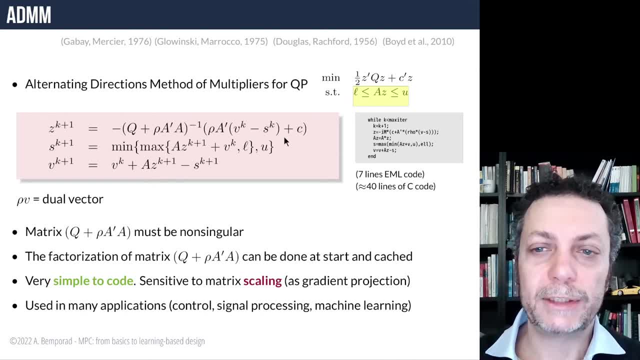 And this is a good algorithm because it's still simple to implement. it tends to be, in practice, fast and also numerically robust. In case of LTI models and in case you don't change the weights in the cost function, these metrics here can be pre-computed offline and cached. 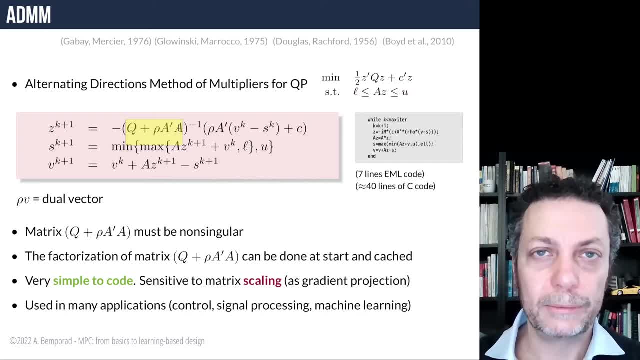 So pre-computed and you can factorize. for example, compute the Chielewski factorization of this metric and store the Chielewski factor in memory to reuse them online for performing the iterations. This algorithm can be sensitive to scaling, so to the way you scale the constraints and also the primal variables. 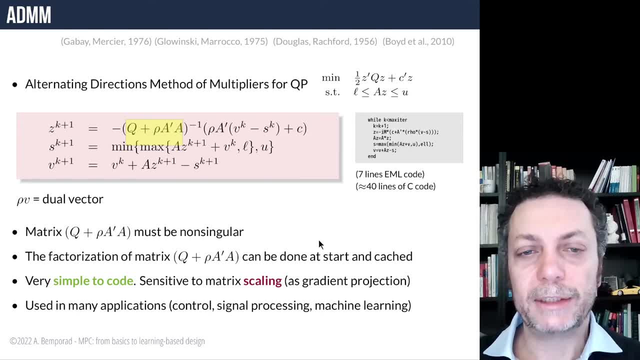 There are some techniques, some preconditioning techniques that can be used. You can change, rescale the problem so that it has better convergence properties that you can show. And this is not only useful for control. it's actually already used in several applications, for example in signal processing, and also in machine learning problems and others. 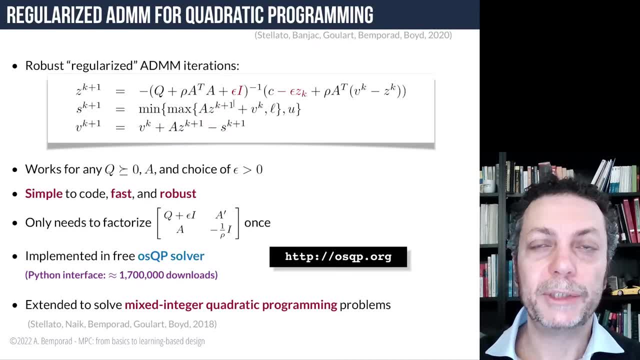 Now a slightly different version of the ADMM or, if you want, a regularized version of the ADMM algorithm is to introduce kind of a proximal point iteration on the z vector where you weight also the difference between zk and the previous value. 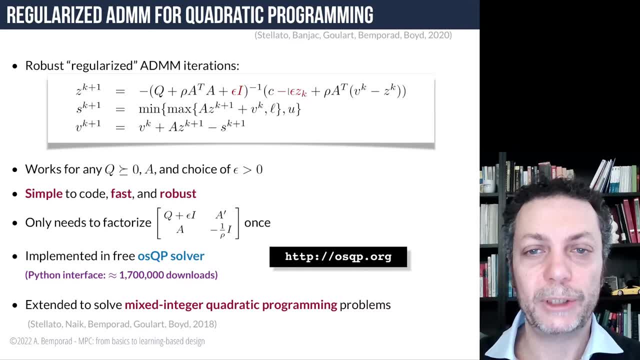 So the norm of this difference is weighted. the square norm of this difference is weighted by some epsilon, which is a tuning parameter of the algorithm, so that the iteration now gets based on the inverse of these metrics, arbitrarily well conditioned by choosing a larger epsilon. 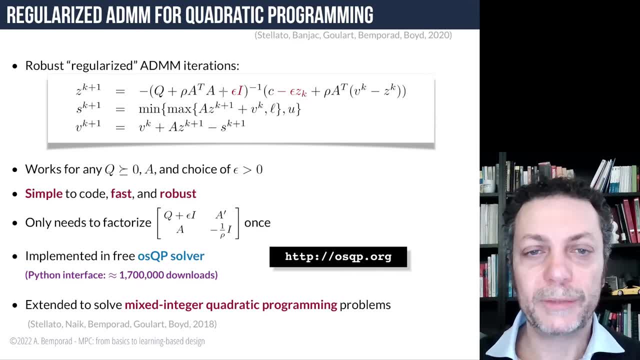 The larger epsilon that's lower is in general the convergence, but you can choose values of epsilon. that makes these metrics well conditioned enough, And you can look at this also in a different split formulation of ADMM. This is what is implemented in the OSQP solver, which is an open source code. 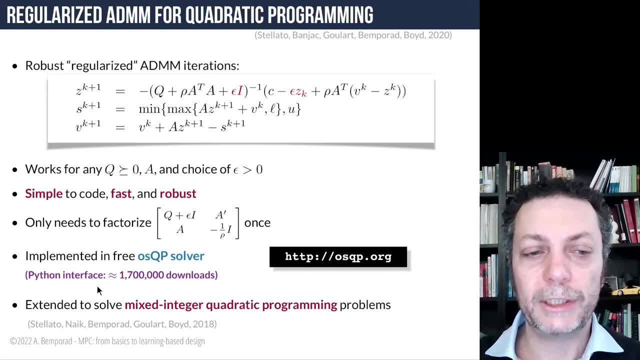 You can download from here. This is used a lot. actually, The Python interface has been downloaded many times. This maybe is not even an outdated number, because it's a simple algorithm and it's quite efficient. Not maybe the best algorithm you can use, but it's quite efficient and robust. 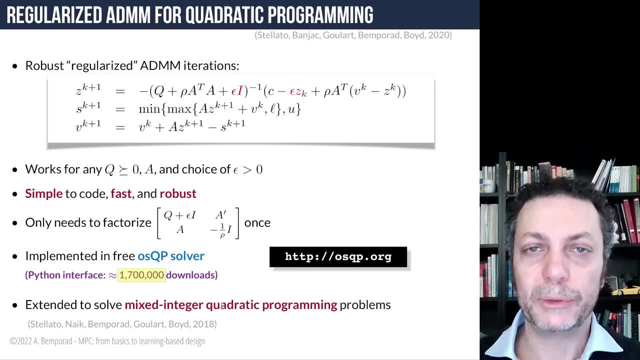 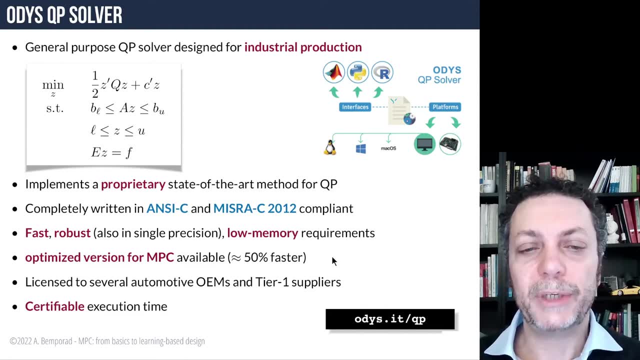 And also, of course, you can use this for mixed integer relative programming problems. Let me also mention another class of solvers based on active set methods, in particular the one that is used by Odis in their MPC software. This is a proprietary code which is based on a proprietary algorithm of the active set family. 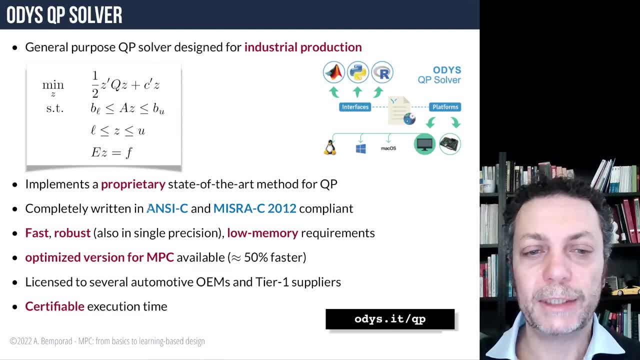 And it's totally written in NCEC and it's MISRA-C compliant so that it can pass through software validation, And it's also used for acceptance in industrial products. What you have from this type of method is that those are extremely fast and extremely robust. 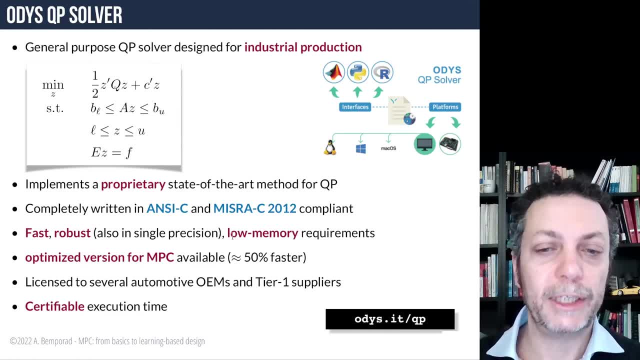 also in single precision arithmetic and they don't take too much memory And they really, according to my experience, they beat at least four QP problems that don't have too many variables- I will come back on this- Say up to a few hundreds of variables and constraints. 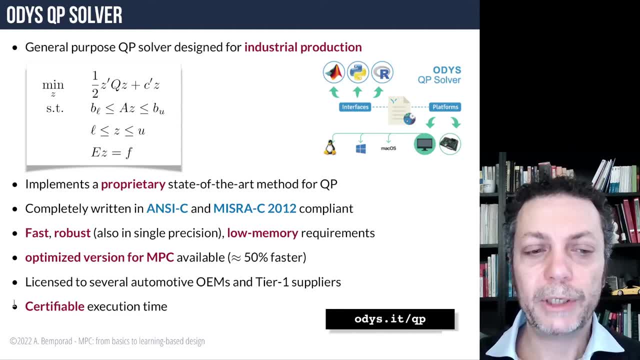 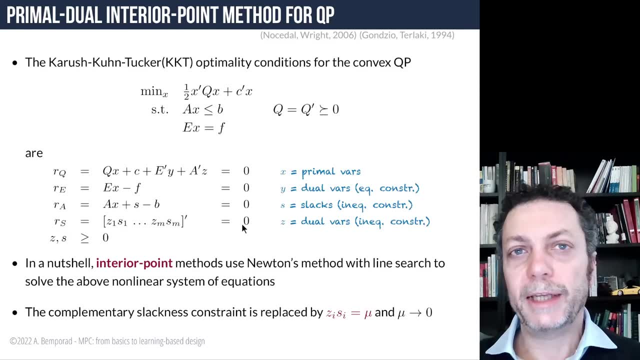 Those really perform well And you can also- I will mention this later- you can- also certify the worst case execution time. Finally, another popular class of methods that are applied in MPC are primal doer interior point methods Where, in a very nutshell, the idea is that you take the problem, write the Karush-Kuhn-Tucker conditions for optimization. 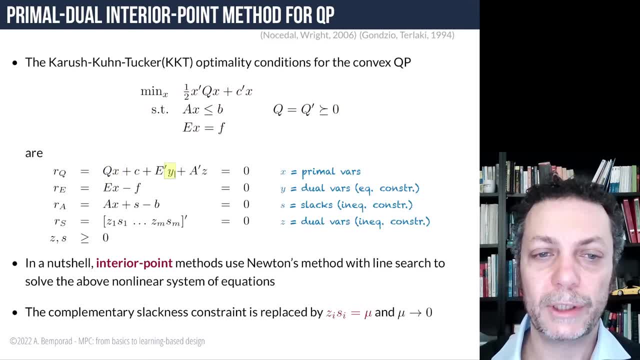 So vector X, together with the vector of dual variables for equality constraints and the dual variables for inequality constraints. They must satisfy a linear set of linear equations. You need feasibility for the equality constraint as well as feasibility for the inequality constraints that are formulated as equality constraints by introducing a vector of slack variables. 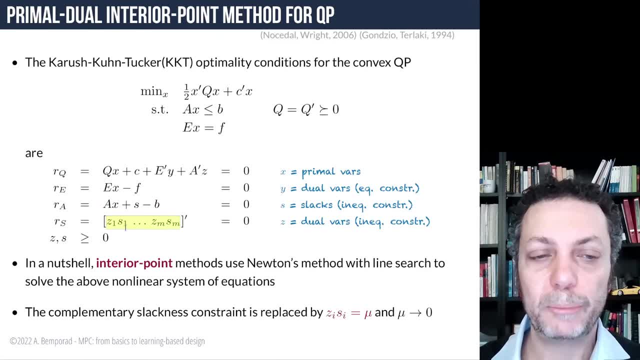 Plus the complementary slackness condition. So each pair of Z S variables their products must be zero, for all the inequality constraints you have in the problem. So the idea of interior point methods is to particular primal doer. interior point method is to use Newton's method to solve this non-linear system of equations. 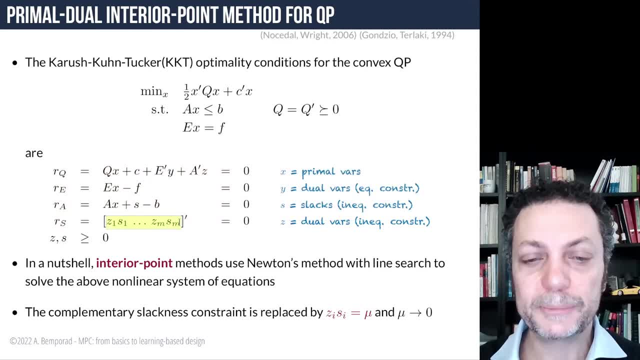 Non-linear, because you have these products here And then do this iteratively using Newton's method, And while doing this you replace the complementary slackness condition with a relaxed version of it, So the product equal to a positive value mu, And then you send mu to zero. 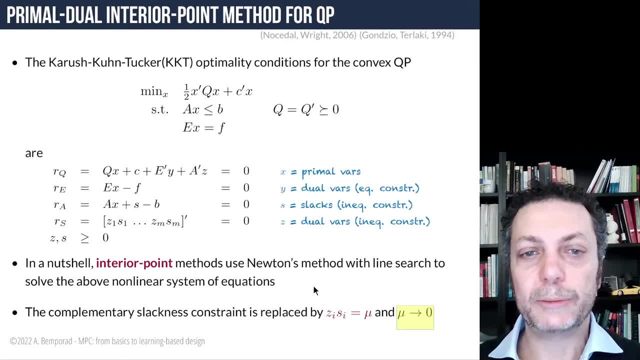 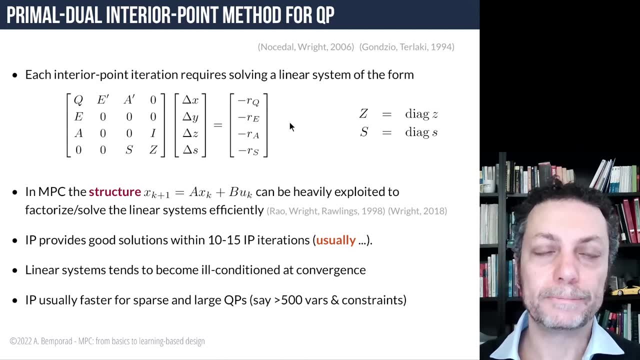 So to converge to a solution, This method has pros and cons. Each Newton iteration requires solving a linear system, So there are good algorithms for solving linear systems. You have to be careful with the linear algebra, because these tend to be ill-conditioned. 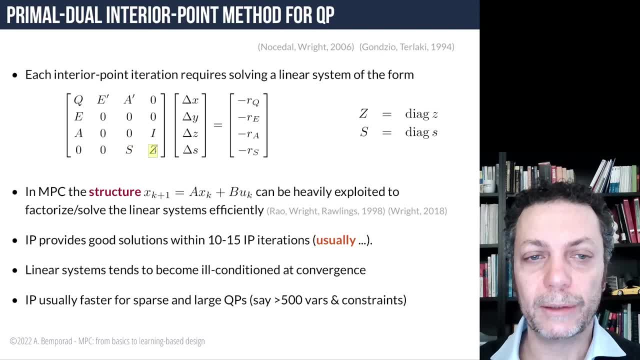 Especially close to convergence because some entries, here or here or both, become zero. Being a Newton method, you can usually get the solution in a small number of iterations, Say 10, 15 iterations. I'm highlighting here usually because this is good for the average case. 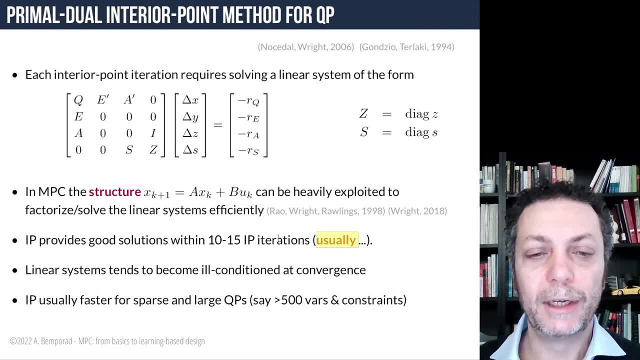 Not so good for the worst case. so it may be hard to estimate what is the worst case: execution time As a function of the vector of state of reference signals. But on the other hand, by exploiting the sparsity of the problem and of the system of equations you are solving. 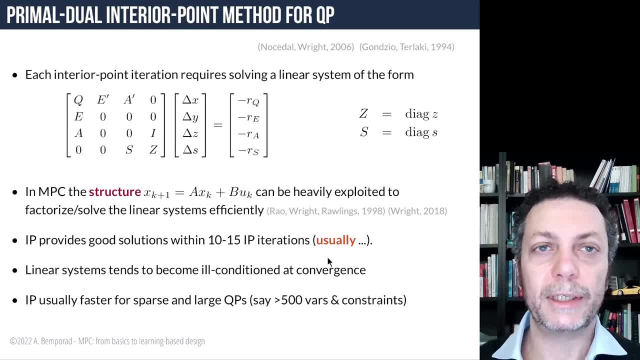 you can be very efficient and actually even exploit the particular structure of the MPC problem, For example, described in these papers here, To make the solution of this linear system very efficient so that this method becomes really good and fast for big problems Where big, say, more than 500 or 1000 variables and constraints. 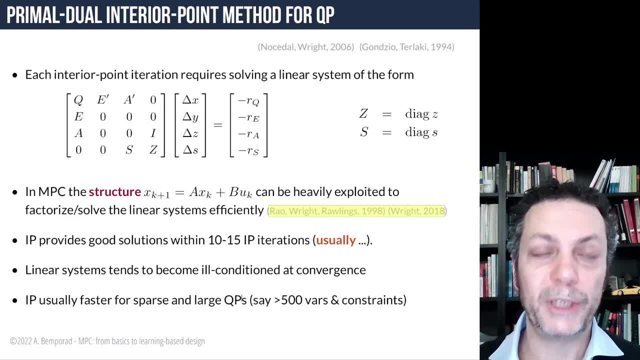 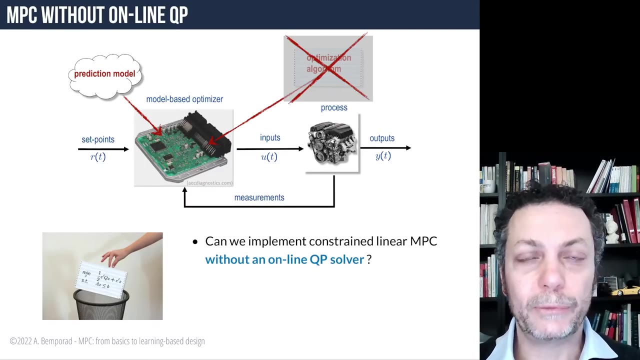 For large-scale QP problems. these are actually the dominating technology Because the other methods tend to be slower. Okay, so this concludes this part on solution methods for MPC And in particular for the quadratic programming problems that arise in MPC. So we have seen different methods for solving quadratic programming problems for implementing linear MPC. 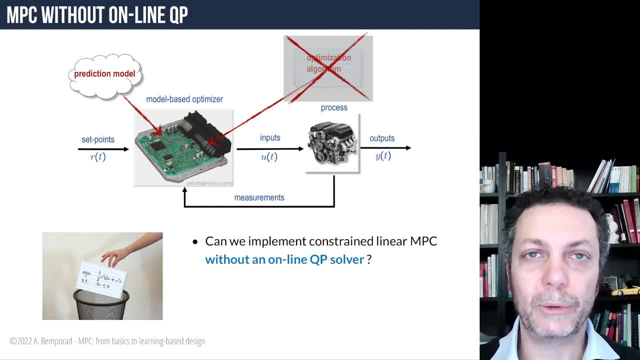 Now the question is: can we implement MPC without a quadratic programming solver? So let's say we are not able to implement a piece of software code that solves a QP in our control software, Can we still apply ideas of MPC? Well, the answer is yes, we can do that. 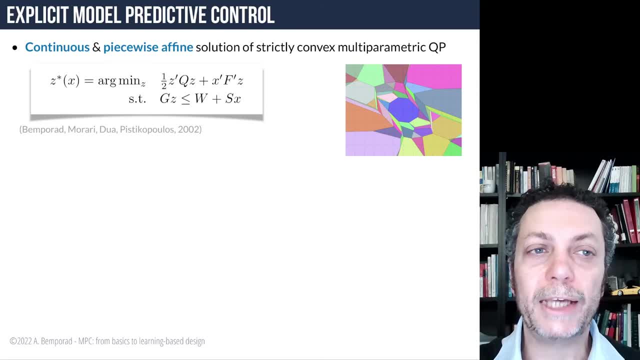 And the idea is to use what is called explicit, moderated predictive control. So look at the quadratic programming problem as a multi-parametric quadratic programming problem Where the vector of parameters that affects the linear term of the cost function and the right-hand side of the constraints 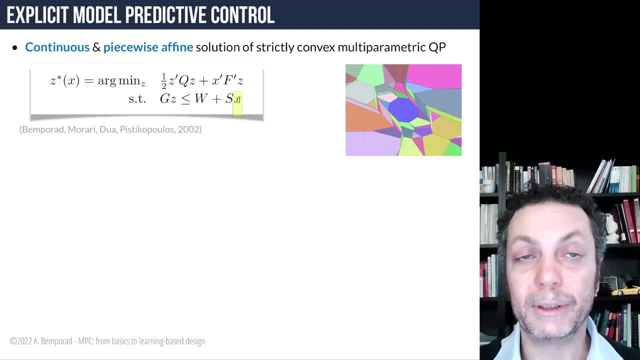 will be our state vector. reference past input, even upper-lower bounds on the input and output variables, And try to solve this problem offline to get the optimizer z star as a function of this parameter vector. Now it turns out that the solution for this problem can be shown that is continuous and piecewise, affine. 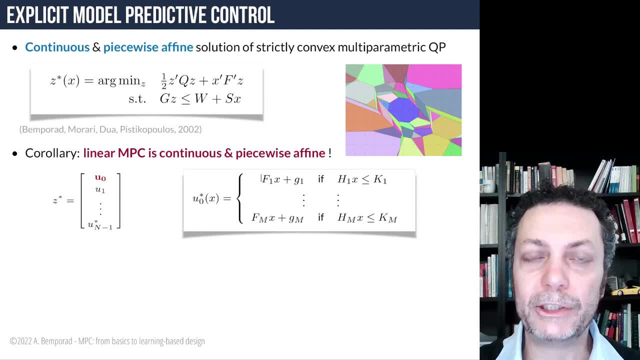 Which means that it can be written as a collection of a linear function of x plus a constant term, So affine functions over a polyhedral partition, as you see in the example here in the picture of the parameter space. So this is the solution. 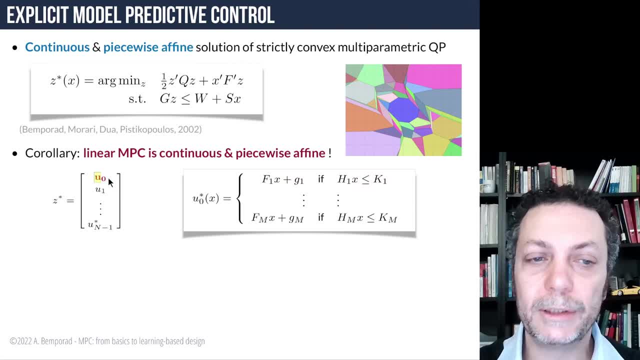 In particular, we are interested in u0, the first component of the solution. So the control law that we are applying is actually a continuous, piecewise affine control law. So this provides an alternative way of implementing the controller. It actually provides an interpretation of what you are doing. 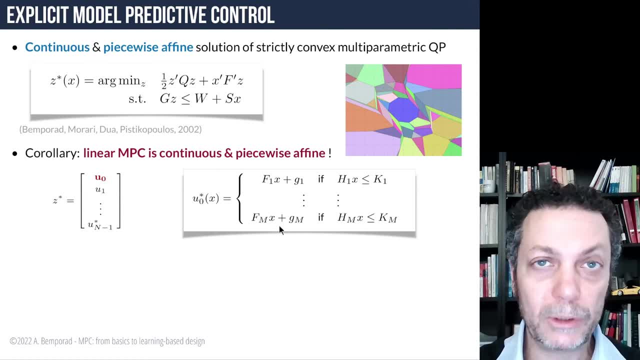 Even if you are solving QP problems online, you know that you are implementing implicitly a piecewise affine control law, And this has been investigated by different people. This is a paper we published back in 2002 together with Manfred Morari. 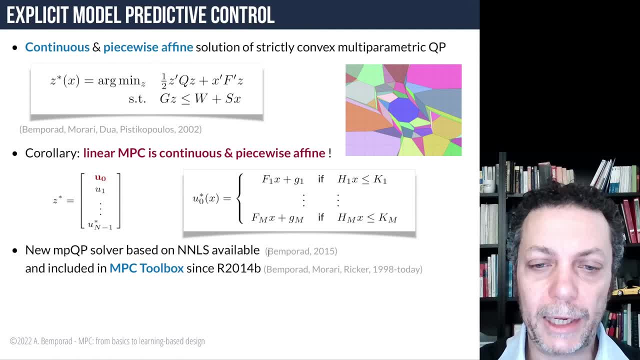 On this. there have been other papers by other authors. I implemented a new method some years ago for solving MPQPs, based on non-negative least squares for solving the geometric computational problem. Geometry involved in constructing the solution Which is now. I'm mentioning this here because now this is part of the model predictive control toolbox. 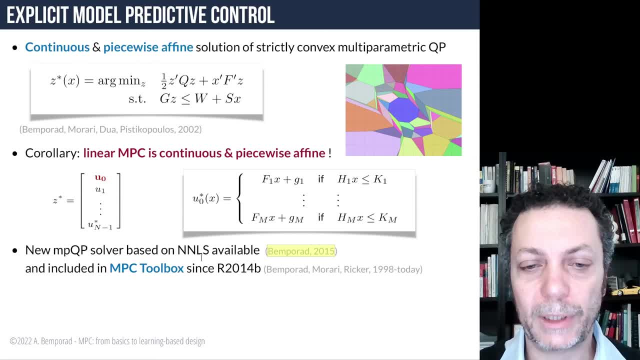 This is built by the Matworks since 2014.. However, the question is: we have a different alternative Now. when is explicit MPC better than online QP? This number of polyhedral cells tends to grow exponentially, Especially with the number of constraints you have in the problem. 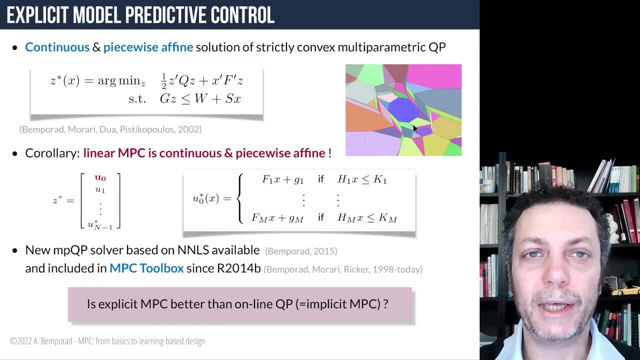 So in principle it's a good idea, but in practice it may bring a lot of regions or a lot of memory to store all the regions And even a lot of flops to evaluate where you are in the partition. So solve the so-called point location problem. 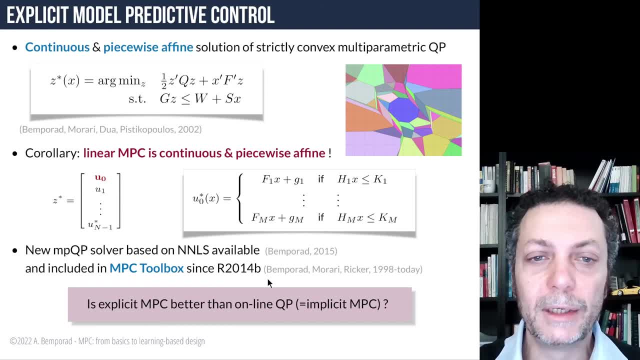 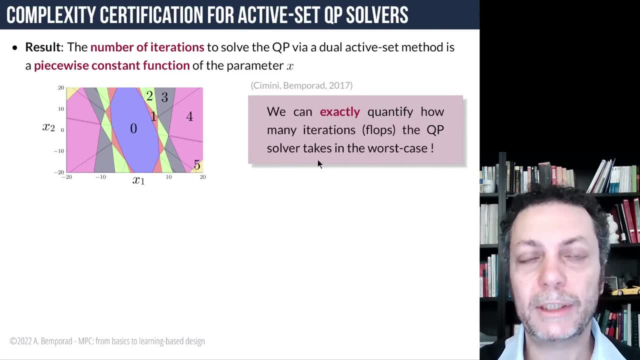 And then evaluate the control law. So to analyze this and to answer this question, actually exactly Together with Jonathan Cimini, We analyze the behavior of an active set method for QP And show that the number of iterations that the QP solver makes is a piecewise constant function of the parameter vector x. 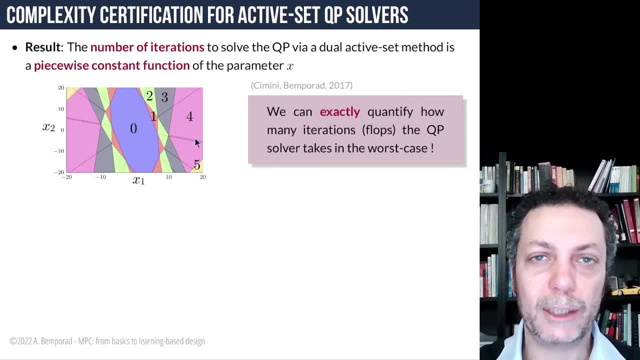 So this is an offline analysis Which requires some machinery, Similar to what you use in explicit MPC. But this is just to analyze how many iterations the QP solver will make. So, for example, in this picture here, The QP problem that we have analyzed. 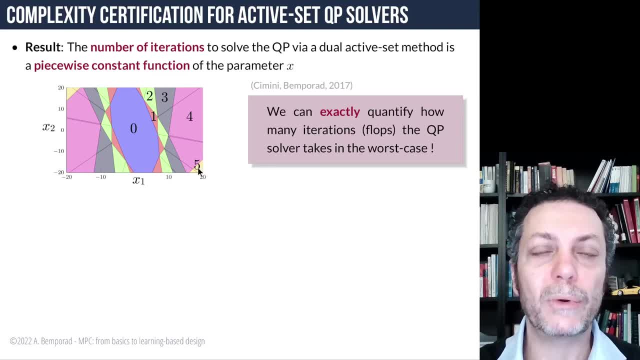 The answer is five. So it will make at most five active set iterations. Actually, we make no iterations here In the purple region. the unconstrained solution is already optimal. Then one, two or three or this yellow arrow will require five active set changes to get to the optimum. 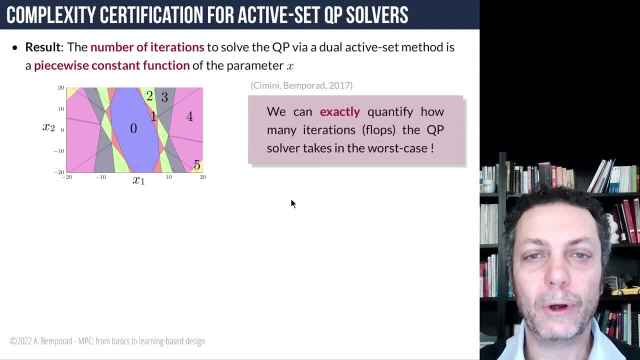 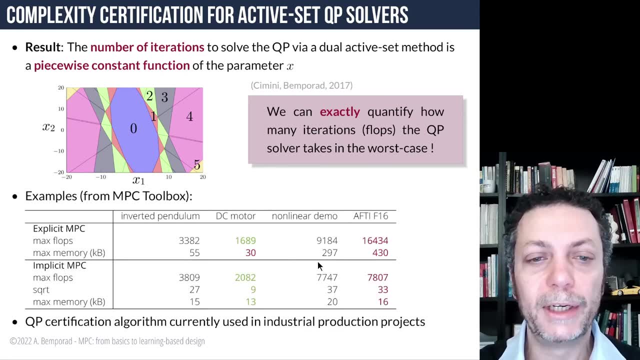 So in this way you can exactly quantify the number of flops that the online QP solver will make in the worst case, And so you can compare. So here we took some demos in the MPC toolbox And you can compare explicit MPC and online. 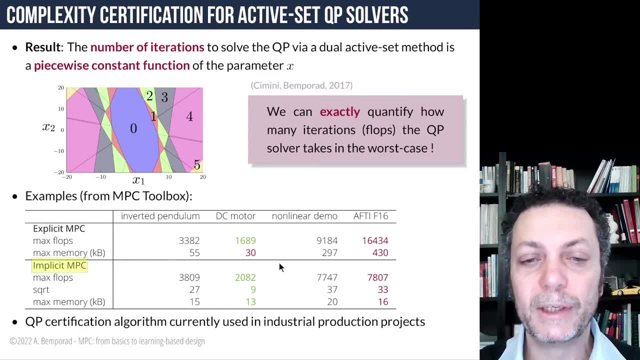 Or, if you want, implicit MPC controller implementation, For example in this DC model. example: In the worst case explicit makes about 1700 flops, While solving the QP online will make about 2000 flops. So worst case difference Memory allocation here. 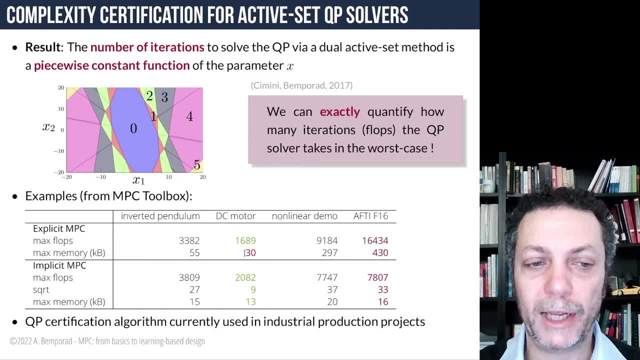 Is smaller with online QP than offline Because you don't have to store the partition, Just the QP matrixes and the QP code, While if you go to other example, For example here, This is an aircraft multivariable 2x2 control problem. 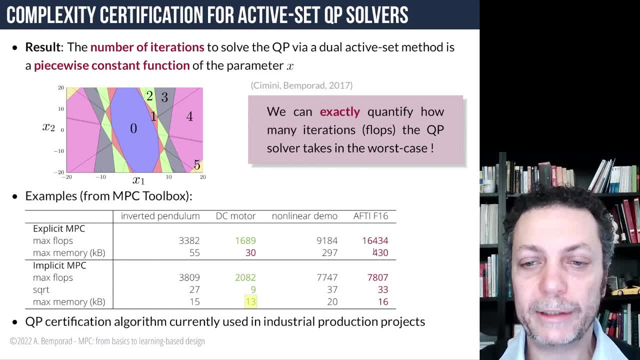 You can solve for explicit MPC. This will require 430 kilobytes of RAM to store the partition And 60000 flops in the worst case, While online QP about less than half of the number of flops And some square roots for the online implementation in the worst case. 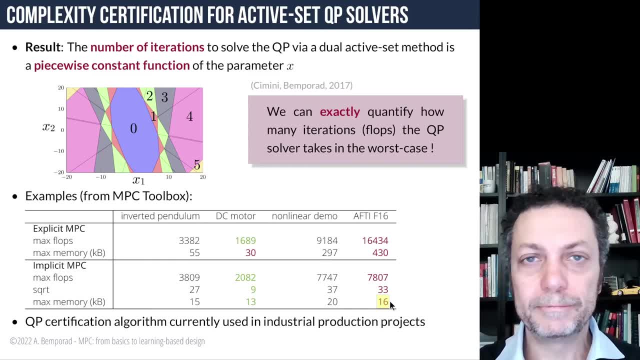 And a much less memory occupancy, So you can decide whether you want to go for one or another. And this type of certification algorithm are actually using some industrial project Really to understand what is the worst case execution time And whether it's worth to go for explicit or not. 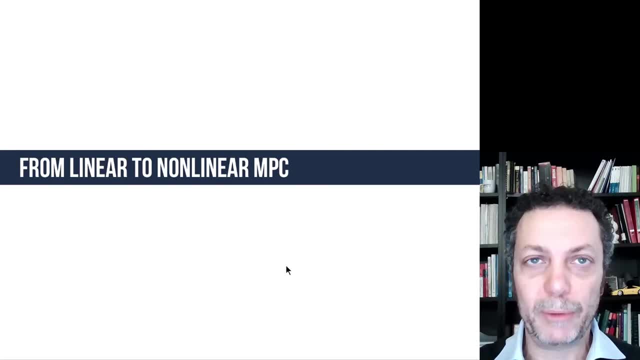 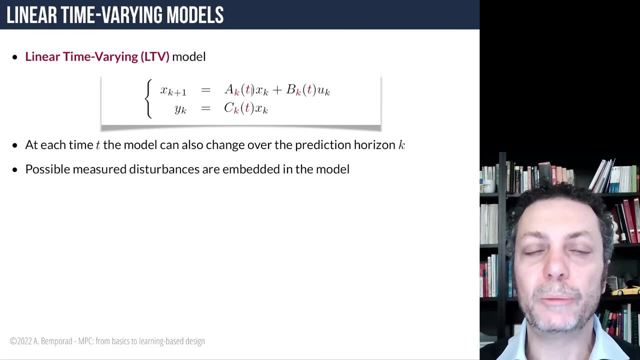 Now, so far we have seen formulation for linear time invariant models. What happens if we have time varying model, For example, this could be periodic systems Or system that change over time, For example because we are, as we will see, linearizing A non-linear model at different operating points. 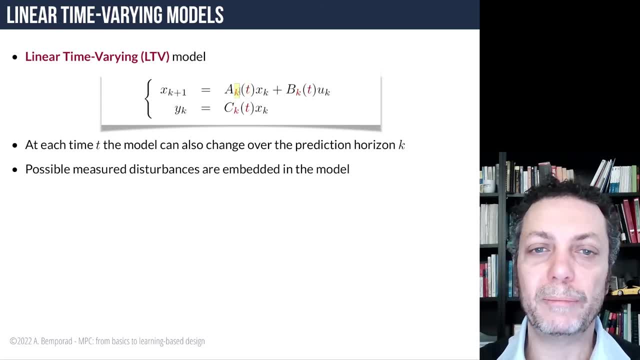 And where we can also assume that the matrixes of the system change over the prediction horizon. So you may have a preview on the way the model changes, For example if you linearize around a non-constant trajectory. So the idea is exactly the same as we have seen before. 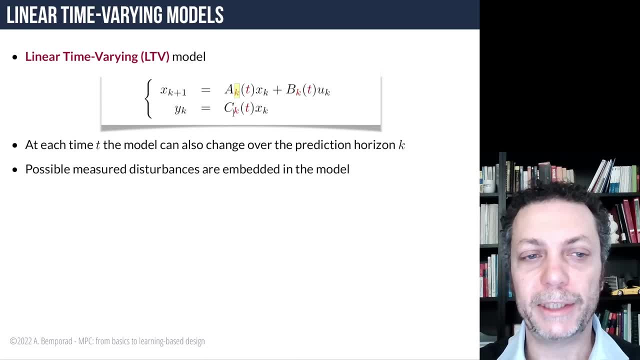 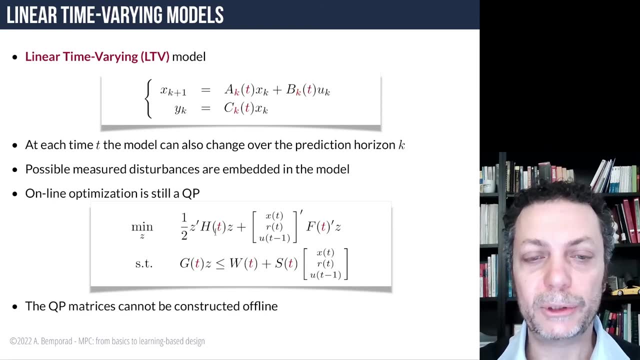 So now handle a linear time varying model rather than LTI. The construction is exactly the same, So you end up in a quadratic programming problem Which has the same structure as we have seen before. The only difference is that the H matrix, as well as the other problem matrix. 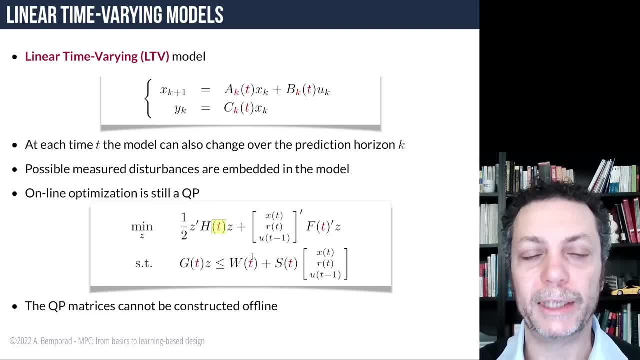 They all can change over time, So you cannot pre-compute those matrixes offline as in the LTI case, But you still end up with a quadratic programming problem. So you can use any of the QP solvers that we have seen before. 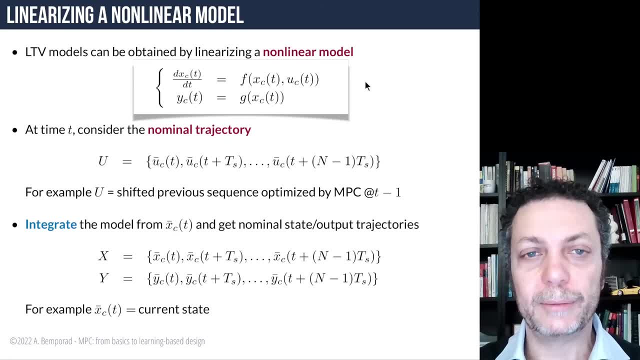 Now in case, the particular interesting case When the model comes from linearization, Let's consider what will happen if we start with a non-linear continuous time model Where, for simplicity, let's assume, there is no input output feed through, So what we can do is consider a nominal sequence of inputs. 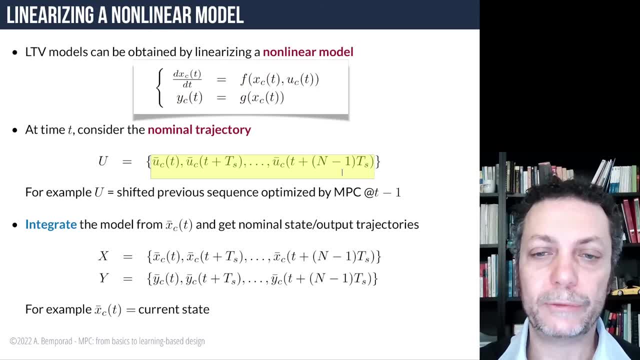 This could be a constant or a time varying sequence, For example, the sequence that we have optimized at the previous time step, And then starting from the current state or from the reference state or any other state Nominal state- you can consider, for example, a steady state state. 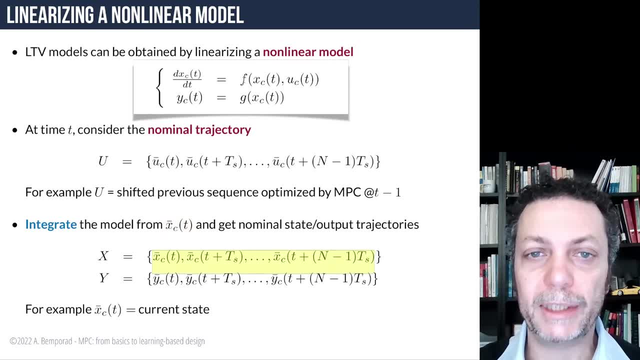 You can build a prediction of the states by integrating the non-linear model. So this is the state that results by starting from the nominal state at time t And applying the nominal input sequence that we have fixed, And you will get also the corresponding outputs. 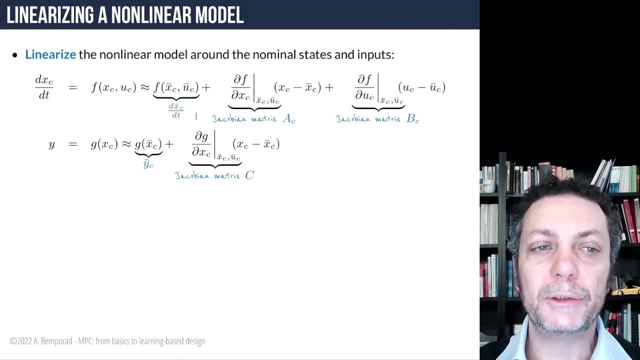 Now what do you do with this sequence? You can linearize the model around those states. So take the non-linear dynamics, Make a first order. Taylor expansion. So this would be the constant term, Which is the vector field for the state update at the nominal condition. 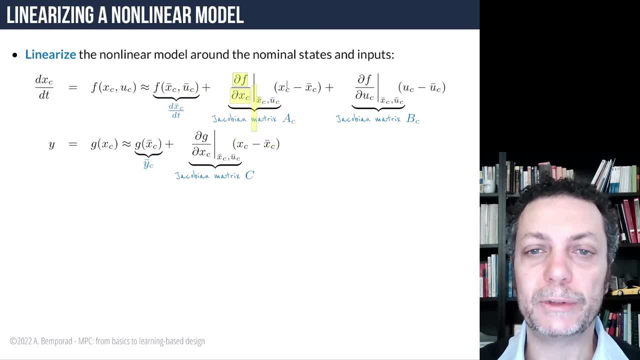 Plus the Jacobian At the nominal state and inputs times the difference between the state and the nominal state And the Jacobian with respect to the input. u times the difference And similarly for the output function. you can also linearize it By taking a first order. Taylor expansion. 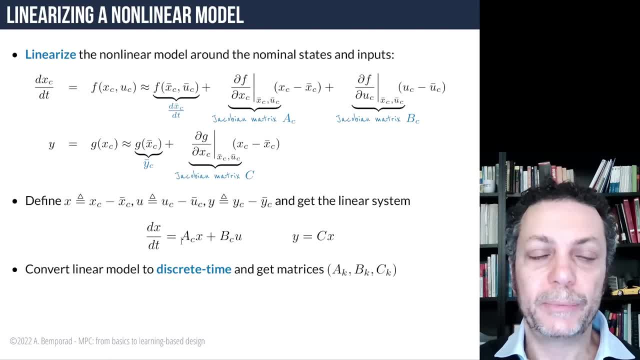 So why doing this? Because we end up with a linear continuous time system If we call x the difference between the predicted state Continuous time and its nominal counterpart, As well as we call u the difference between the input and the nominal input, As well as the output minus the nominal output. 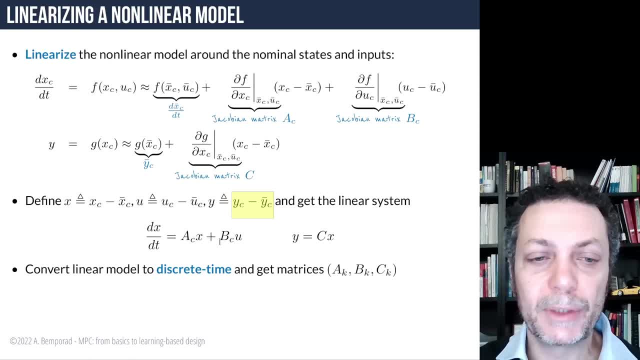 So in this new set of variables the dynamics is linear And we can discretize it. So convert the dynamics to discrete time. To get the set of matrices a, k, b, k, c, k, That we need to construct the quadratic programming problem. Now, this is not the only approach. 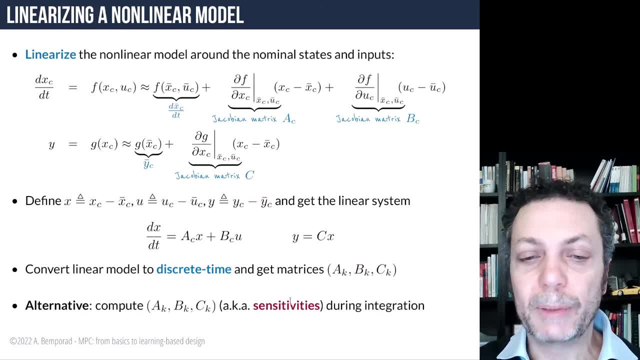 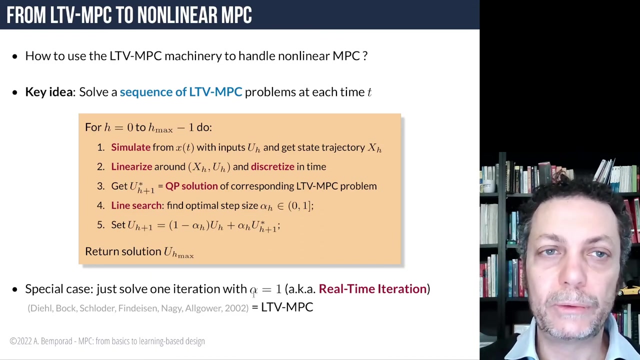 For example, you can, in alternative, build the matrices a, k, b, k, c, k While you integrate the model to get the nominal state and output trajectory. You can treat them as sensitivities during the integration of the model. So how to then combine this linearization to solve non-linear MPC problem? 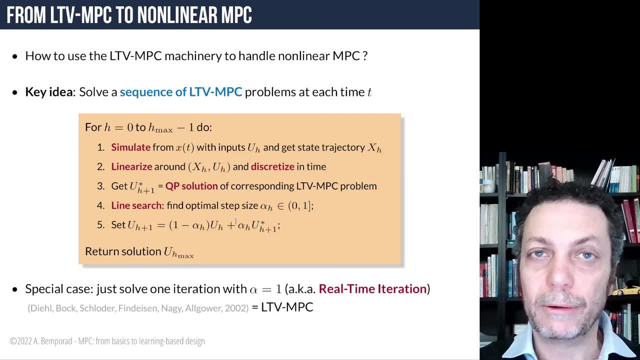 So here is an approach. So let's say, you have built up the machinery to solve MPC problems Based on linear and varying systems, using QP solvers. Now here is the idea: You can, at each time step, solve a sequence of QPs. 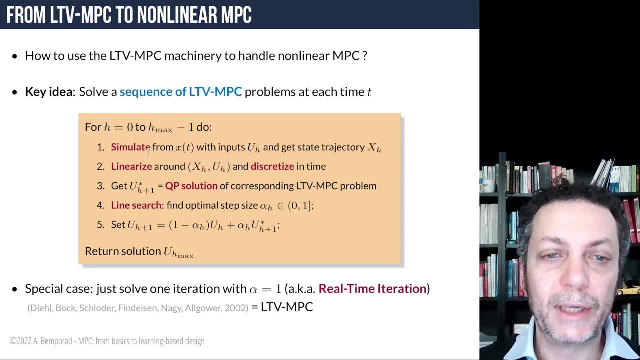 Which is a sequence of linear time varying MPC problems, Where each time you start from a nominal input trajectory- This could be the previous optimal sequence, For example, that you start applying from the current state to get the corresponding trajectory- You linearize and discretize the system, as we've seen before. 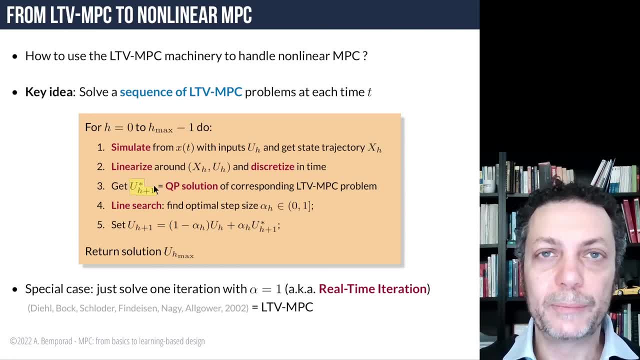 Then solve the QP. What you do get is a candidate sequence of optimal moves. Rather than applying this directly, You can do a line search. So make sure that the cost function for the non-linear problem formulation Is decreasing by choosing a proper step size. 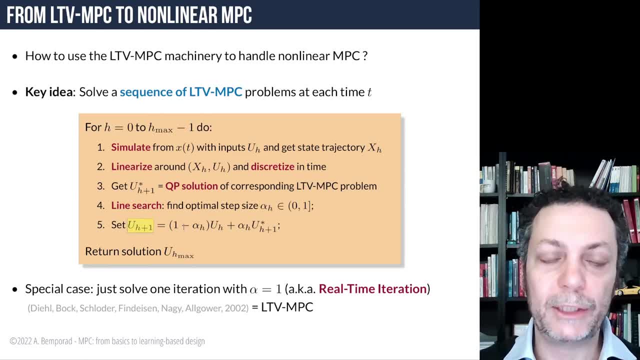 And then update the candidate sequence By taking an alpha step towards the new solution, And then you iterate, So you take this new sequence And then solve another linear time varying MPC problem Where you have linearized now by applying the U sequence to the model. 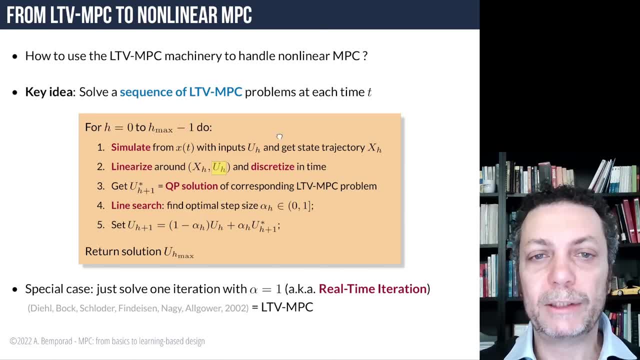 Get the new QP solution and so on. So in this way, by solving this sequence of linear time varying MPC problems, You can actually find a solution for the non-linear MPC programming formulation. Here you can decide to stop Or you can actually run these steps for a finite number- Hmax- of iterations. 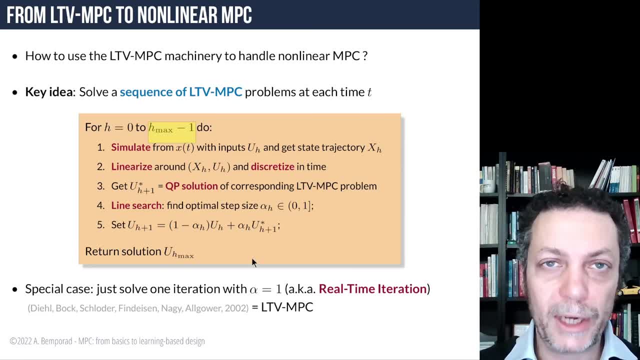 And in particular case when you solve just one iteration And you choose alpha equal one, So you don't do any line search. This is just applying linear time varying MPC And this is also called the real time iteration scheme That was studied by Moritz Dihl and others in the past. 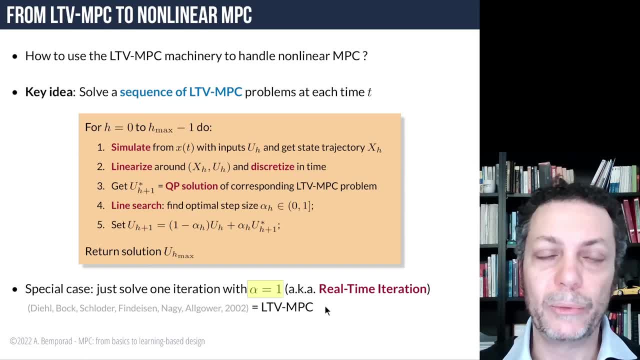 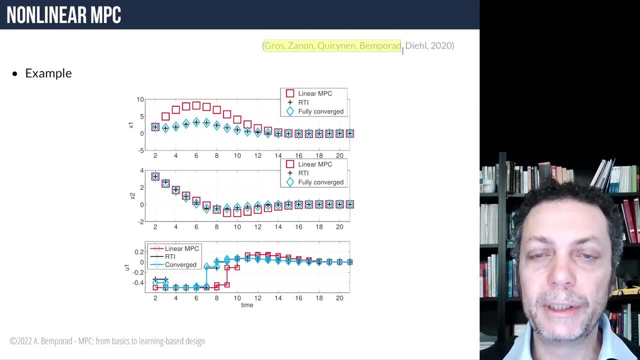 As in a very efficient way of implementing, in a suboptimal way, A non-linear MPC formulation. And here is one example taken from this paper, With Sebastian Gross, Maret Zanon, Remke Rienen, myself and Moritz Dihl. 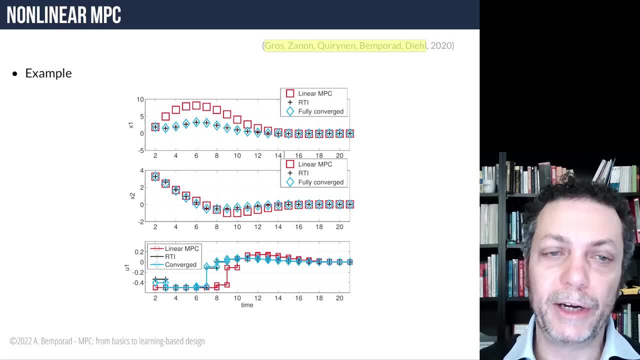 Where we have shown We have studied this relation between linear time varying and non-linear MPC And we actually showed That if you consider the fully converged scheme And compare it to the real time iteration scheme, They are actually usually very, very close to each other. 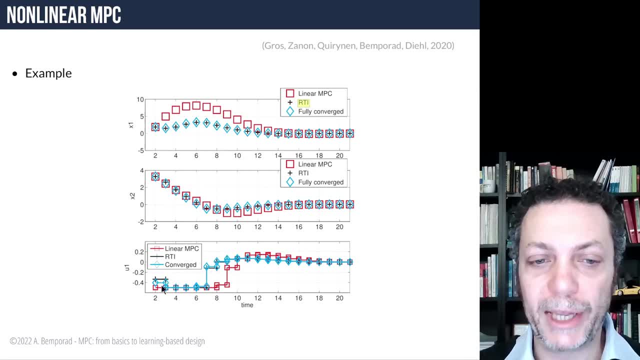 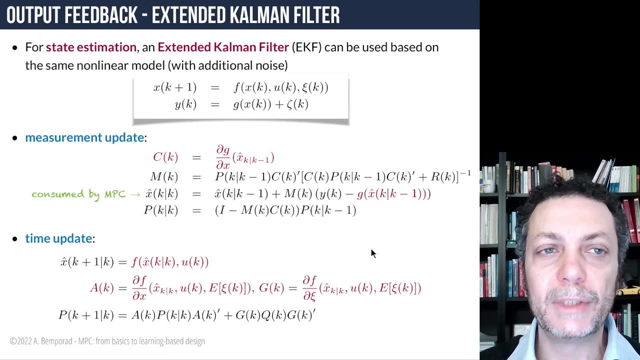 So here you see the difference between the one iteration, which is the black, And the fully converged one, which is the light blue one. It is very close. Now, in non-linear MPC you also have the problem of state estimation. So if you want to close the loop on output measurement, 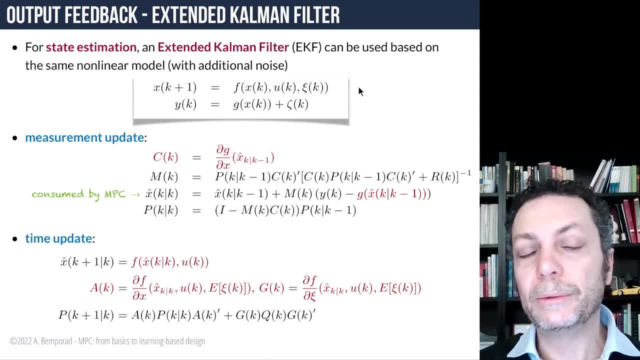 You need a state observer. Typically, what you do is to use a state estimator And in particular an extended Kalman filter. It is particularly appealing because you can reuse the same linearized model you have for MPC To update the filter equations, So the measurement update will consume the output estimation error. 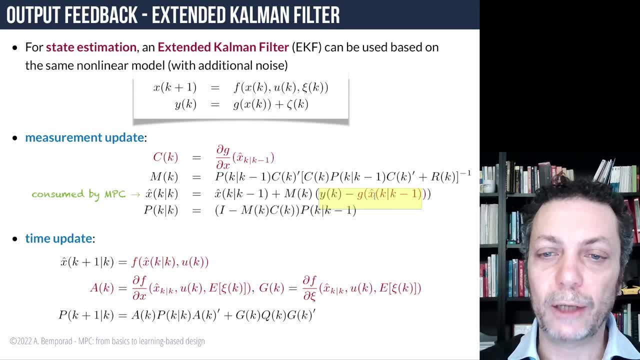 Where you are using here the full non-linearity to predict the output. This will create the state estimate of xk at the current time k That you can feed to the MPC controller to close the loop And then update the state estimate for the next step by using the model. 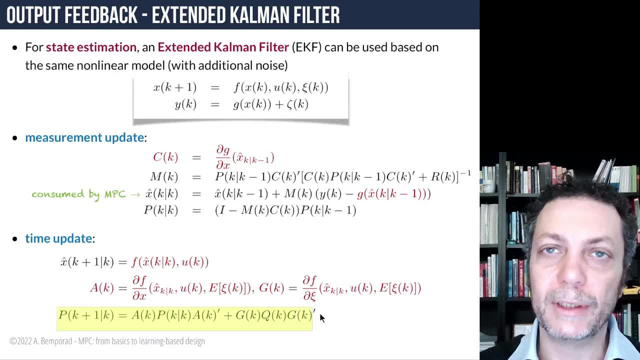 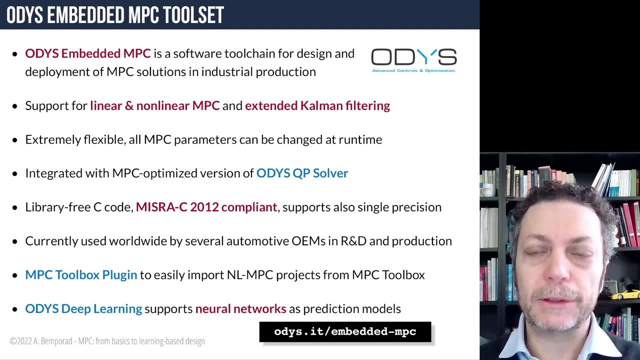 As well as the covariance matrix of the state estimation error, And this type of machinery is at the core of the software tool chain For designing and deploying MPC solutions Developed by the company ODIs. ODIs Embedded MPC Which supports linear, time varying and non-linear MPC. 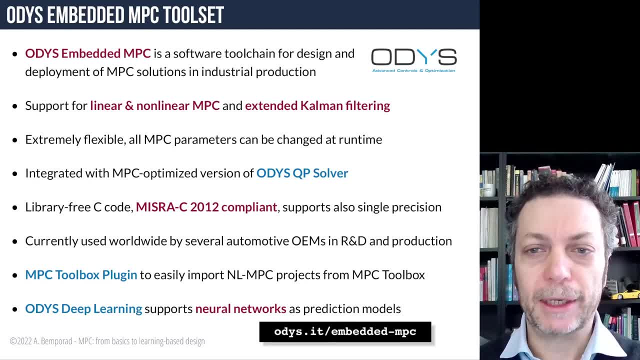 And it has a very robust and fast implementation of the extended Kalman filter Ideas I was mentioning before. And it is very flexible, meaning that you can change all the model equations And the MPC weights And constraints, All the MPC parameters. basically, you can change at runtime. 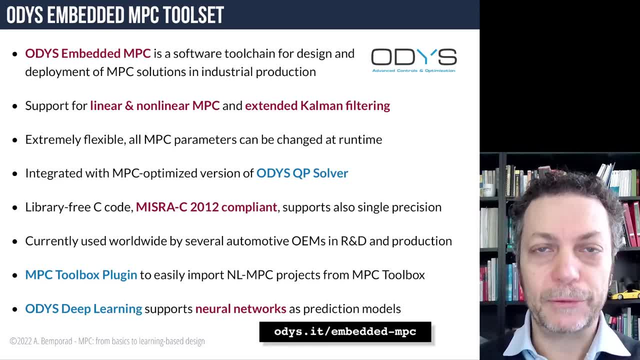 And it's integrated with the ODIs QP solver- Actually with a specialized version of ODIs QP for MPC problems. It's library free, It's written in C, It's MISRA C 2012 compliant And also works well in single precision arithmetics. 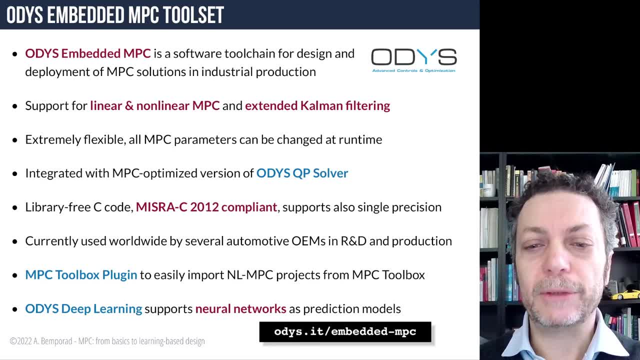 This currently used in many places, Especially by automotive OEMs in R&D and also in production projects, And since recently, also has a plug-in for the MPC toolbox To port designs made with the MPC toolbox, for MATLAB In particular, and non-linear MPC designs. 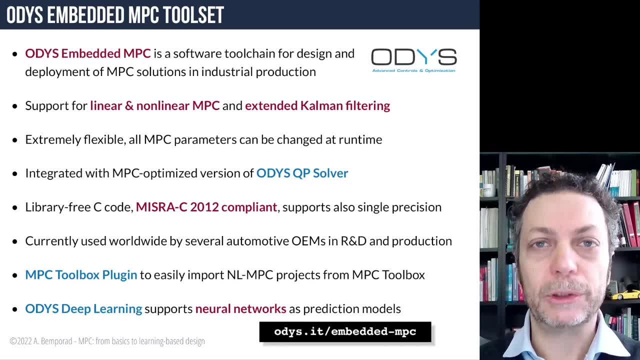 Into the ODIs library to speed up a lot of the execution of the MPC code, And it also has support for neural networks as prediction models, Which is a topic that I will cover in the next part of my lecture.